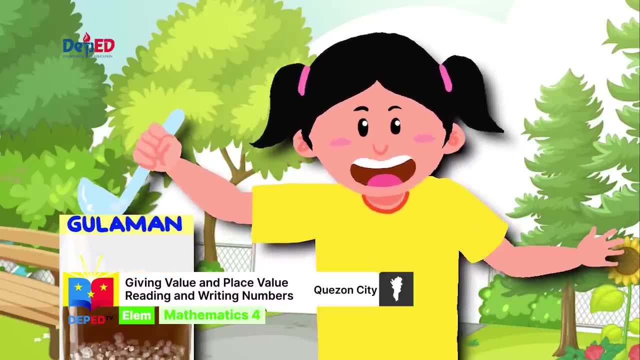 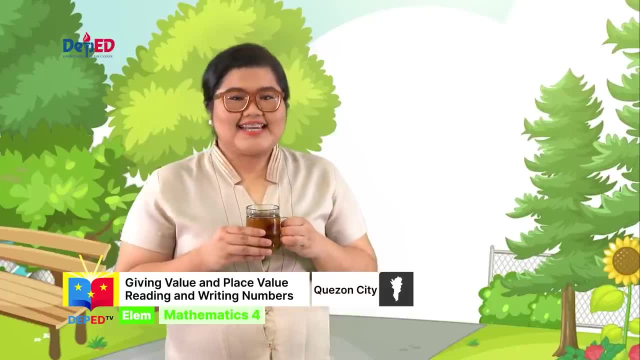 Teacher, I want to help my mom. I want to buy my school supplies using the money I will earn in my gulaman business. Wow, that's great. It will be a great help to your mom in buying your school supplies this school year. 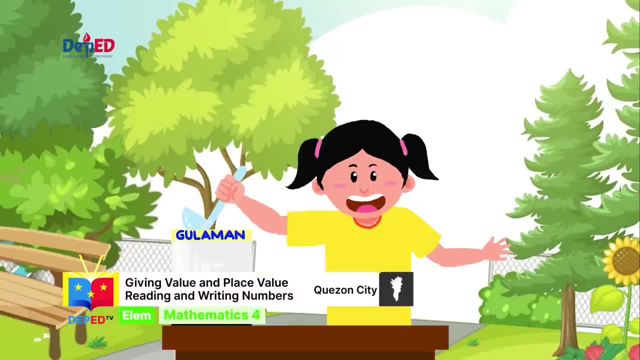 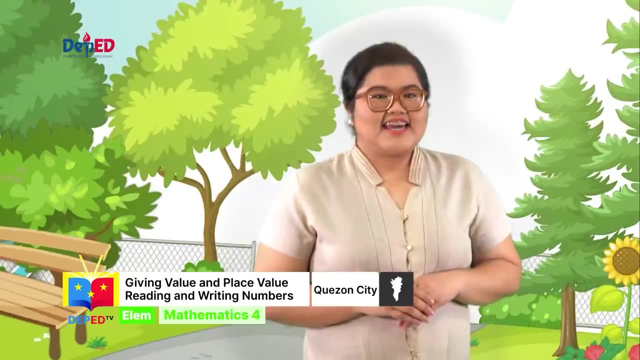 How much money have you earned already? I have earned 816 plus 10.. I have a total of 826 pesos. Wow, that's amazing. Can you remember the amount that Anna earned in her gulaman business? Help me Say it loudly: Yes, she earned 826 pesos. 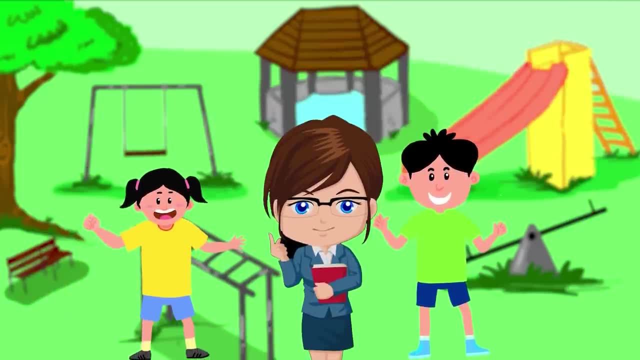 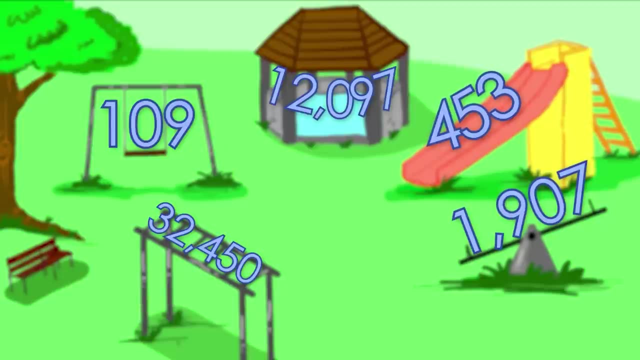 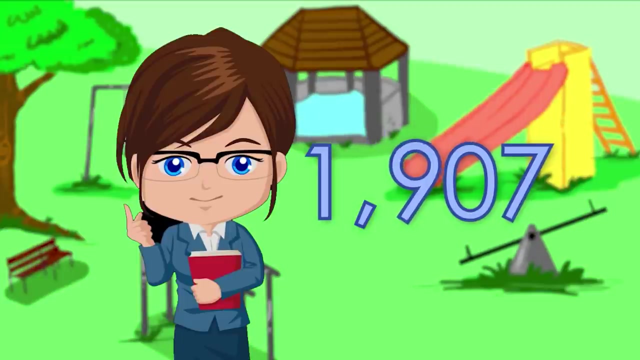 Anna and Tonio, come here, Let's have a game with our Math Galing Buddies. Anna, Tonio, help me read these numbers. Math Galing Buddies. help me read these numbers. Number one: 453.. Number two: 1,907.. Number three: 32,450.. Number four: 109.. And number five: 12,096.. 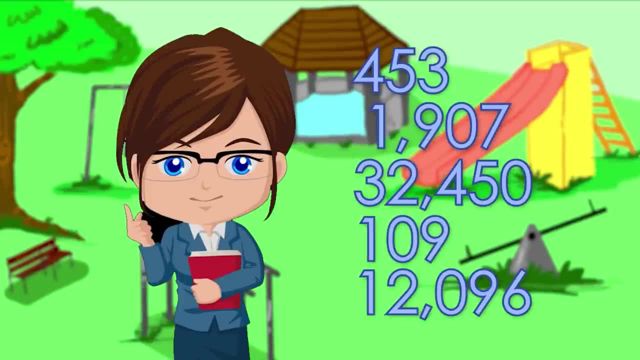 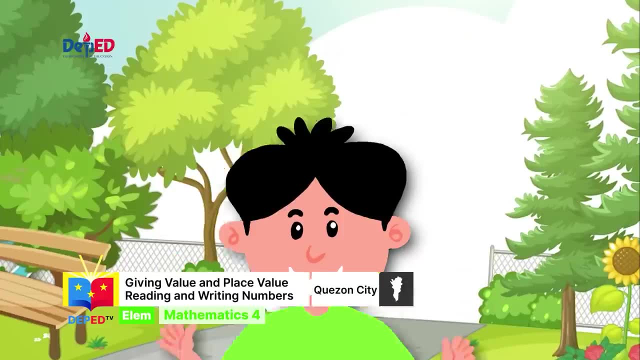 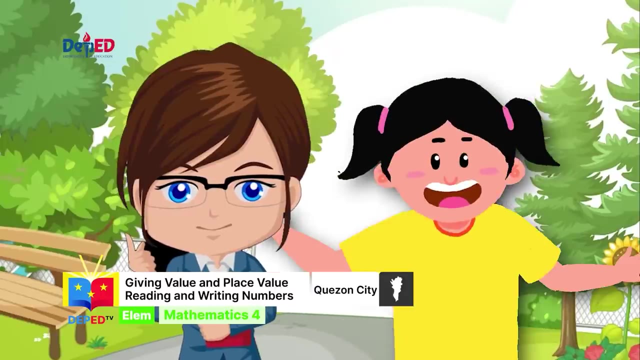 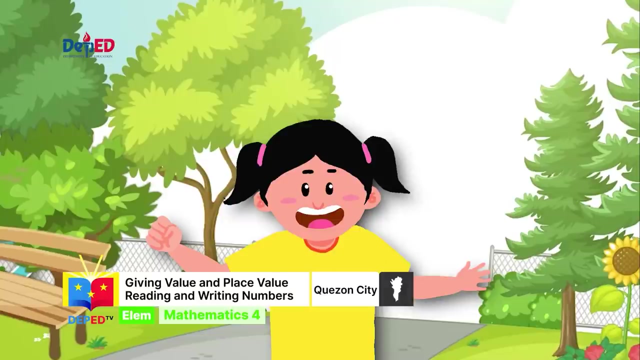 Thank you for playing with us. my dear Math Galing Buddies Teacher Marian, look at Anna. She looks sad. Come let's go and ask why she is sad. Anna, why are you sad? Teacher? I have a problem. I can't remember how to read numbers. 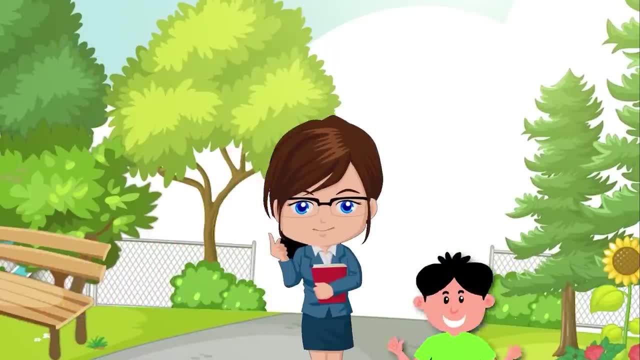 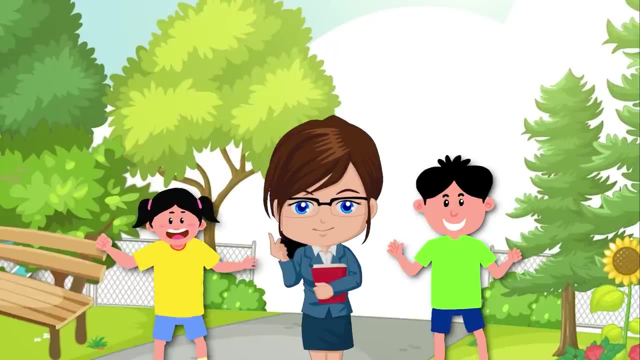 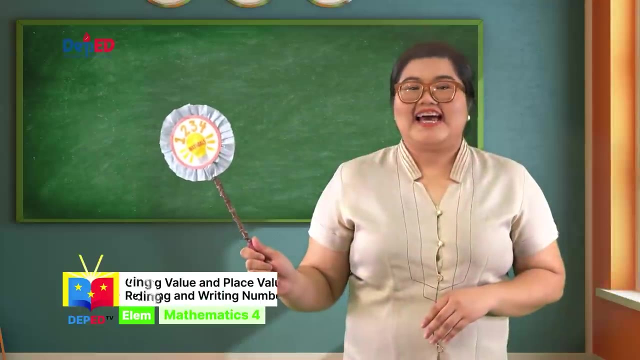 Oh, we are here, Tonio, and our Math Galing Buddies are willing to help you. Let's help you read these numbers. Hop in, Let the adventure begin. We have three magical steps in order to read numbers up to hundred thousands. 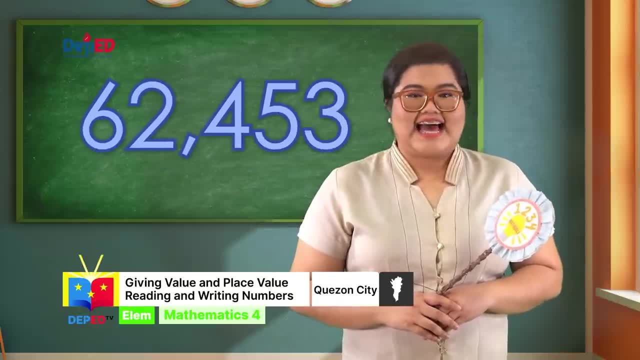 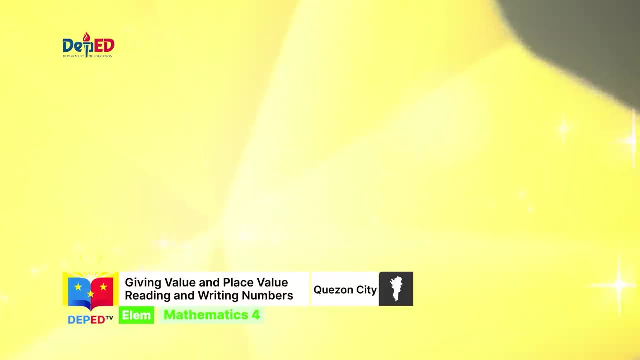 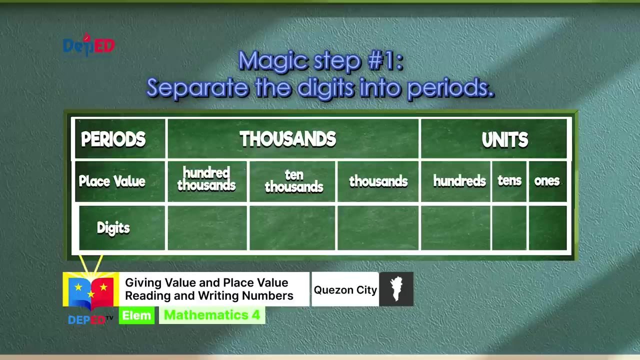 Let us take 62,453 as an example. Magic step number one: Separate the digits into periods. Let's review the place value chart. There are three rows, Periods, place value digits. Periods are thousands and units Under units. there are three place value. 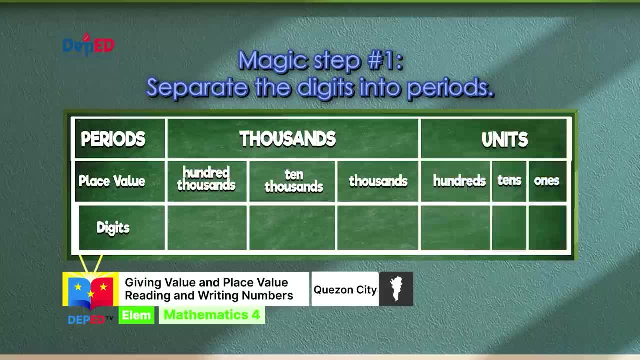 Ones, tens and hundreds Under thousands. there are three place value: Ten thousands, hundred, thousands. The place value of three is ones. The place value of five is tens. The place value of four is hundreds. The place value of two is thousands. The place value of six is ten thousands. 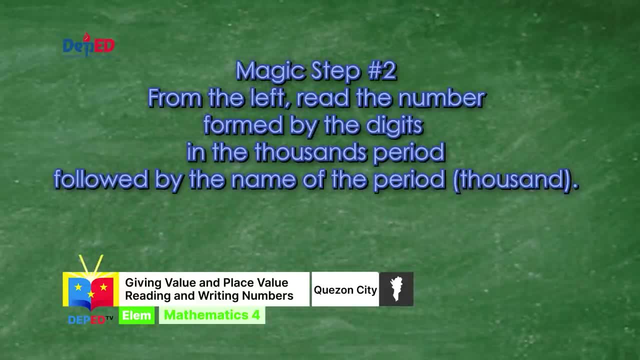 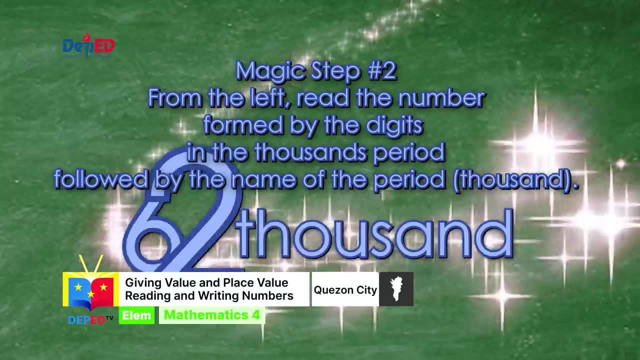 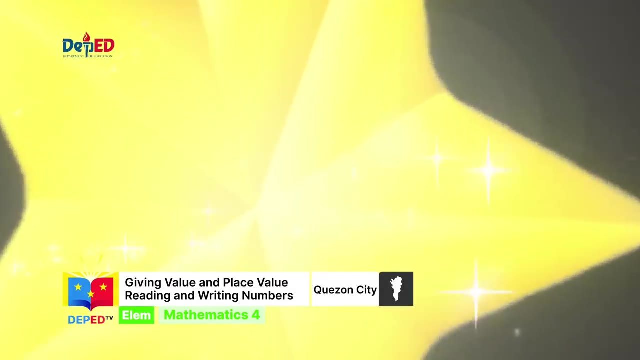 Magic step number two, From the left. read the number formed by the numbers. Read by the digits in the thousands period, followed by the name of the period. Sixty-two thousand Magic, step number three. Do the same with the units period without saying the name of the period. 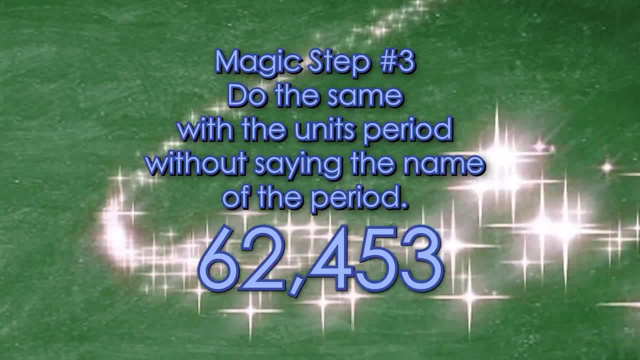 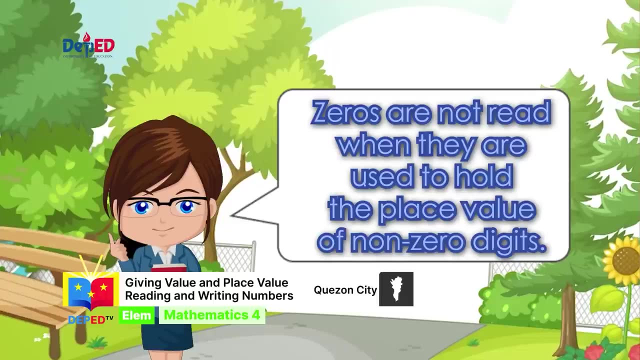 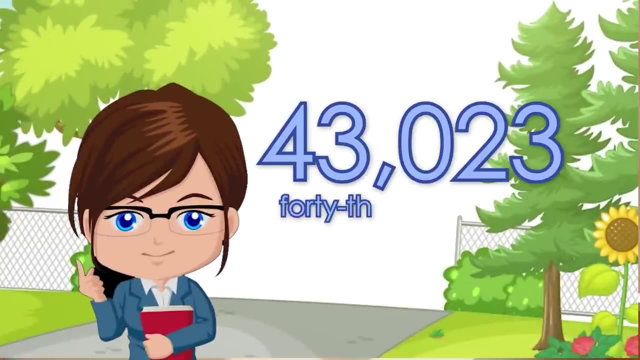 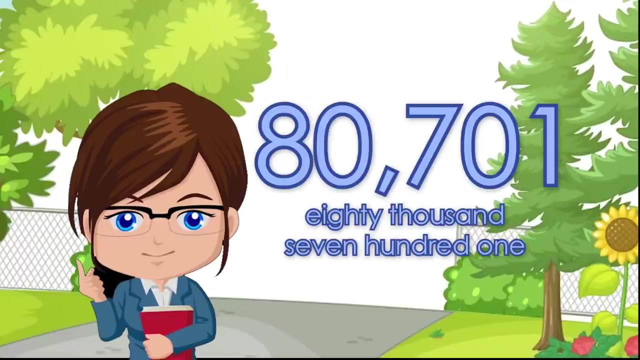 Sixty-two thousand four hundred fifty-three Zeros are not read when they are used to hold the place value of non-zero digits, For example, forty-three thousand twenty-three, Eighty thousand seven hundred one. Oh teacher, Now I understand how to read numbers. 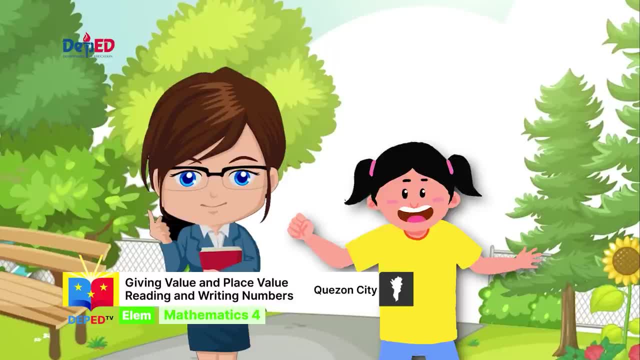 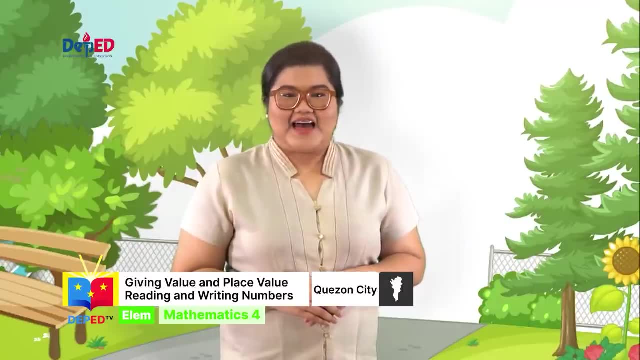 I am excited for our next math-amazing activity. You guessed it right Very good, Anna. I am happy that Tonio and I are good at math And your Math Galing Buddies helped you to read numbers. Let us go back to your classroom and we will have a math-exciting activity. 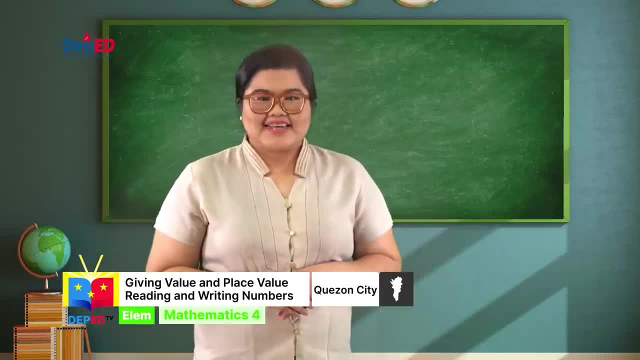 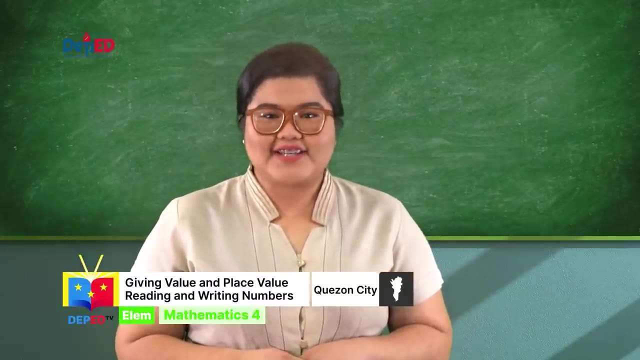 Welcome back. Math Galing Buddies, Math Galing, Math Galing, Math Galing- Practice time. Always remember: as long as Teacher Marian is with you, you can do it. I will give you twenty seconds to read the following numbers. 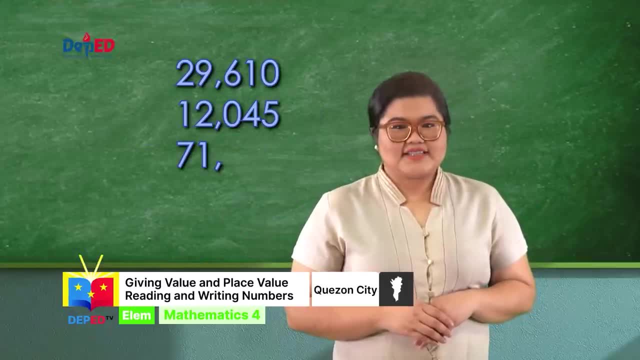 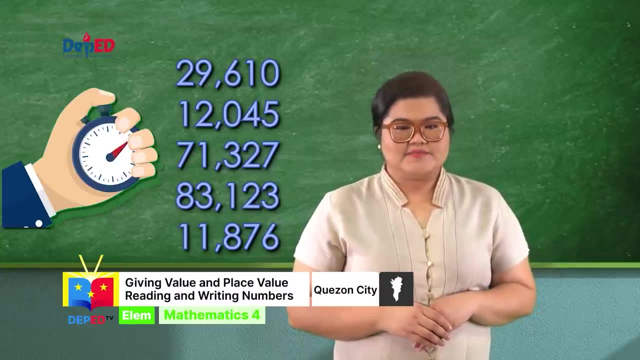 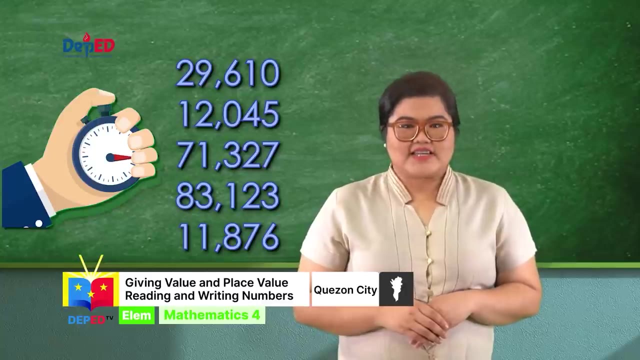 Ready. Twenty-nine thousand six hundred ten Twelve thousand forty-five Seventy-one thousand three hundred twenty-seven Eighty-three thousand one hundred twenty-three Eleven thousand eight hundred seventy-six. Very good, Teacher, Marian. is that you? 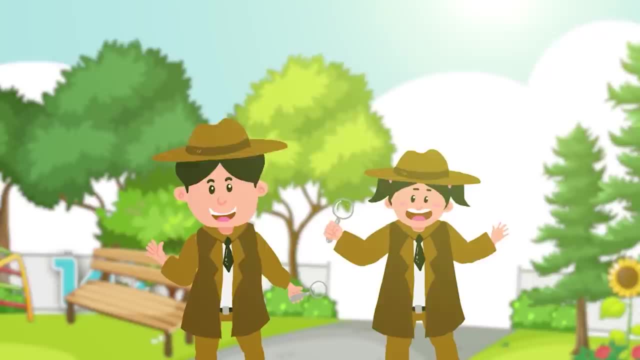 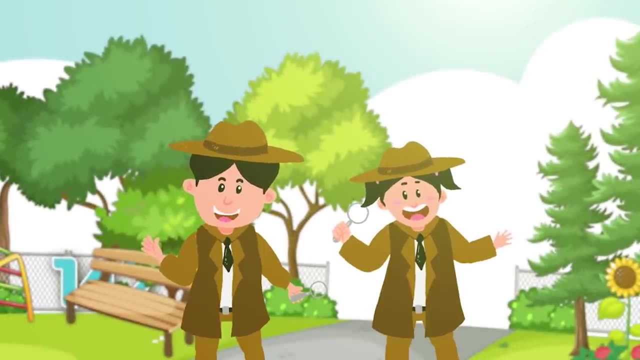 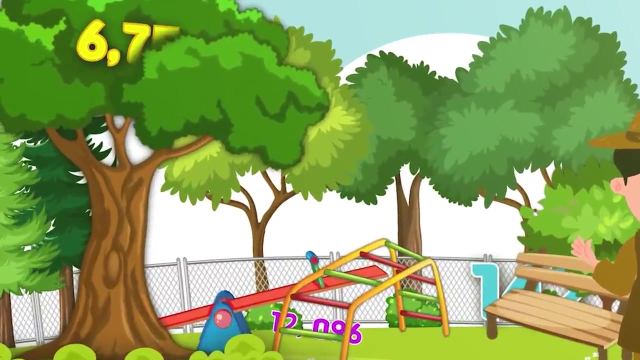 Is that you? Yes, it's me, Together with your Math Galing Buddies, you have an important task. You need to find three given numbers around the playground. You have thirty seconds to write it on your paper Ready. Yes, of course. 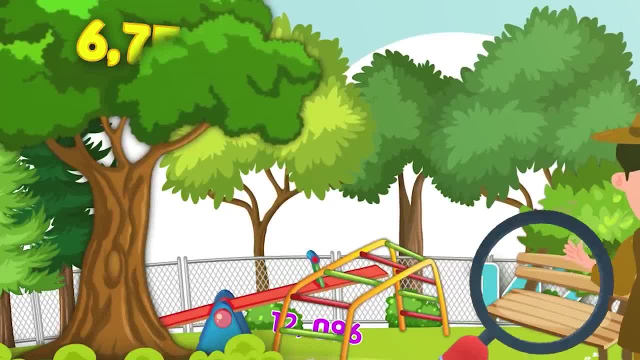 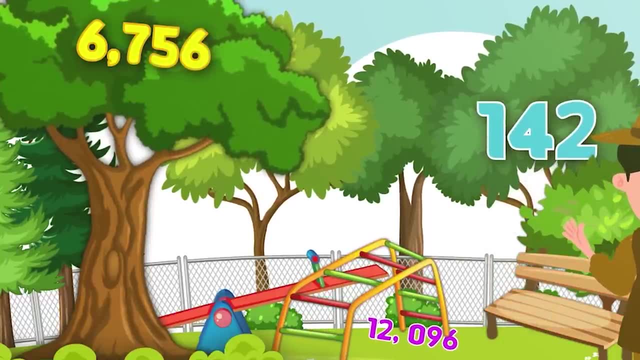 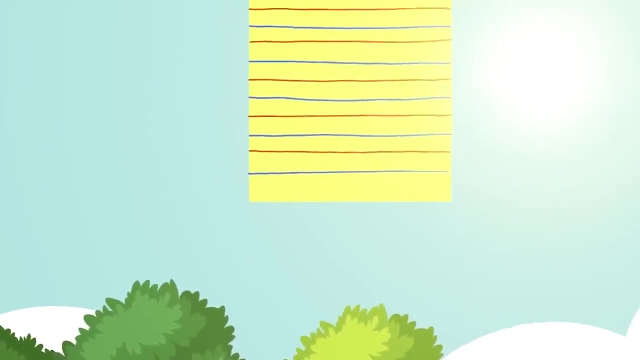 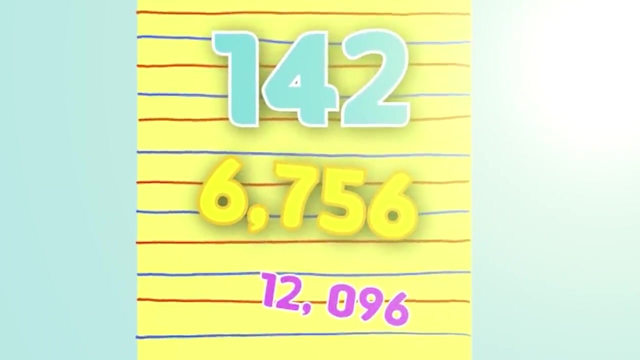 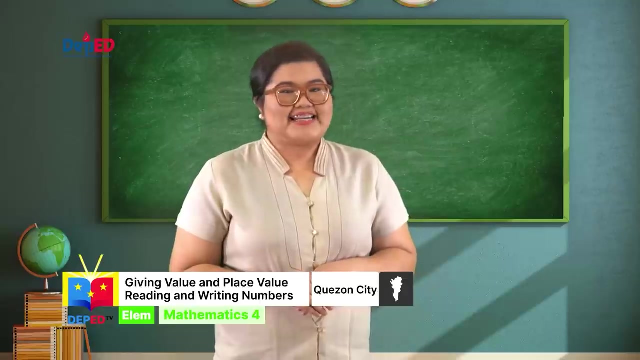 What are the numbers that you have seen around the playground? Six thousand seven hundred fifty-six, One hundred forty-two, Twelve thousand ninety-six. What you have written are numbers in standard form. Standard form are numbers written in numerical form or in digits. 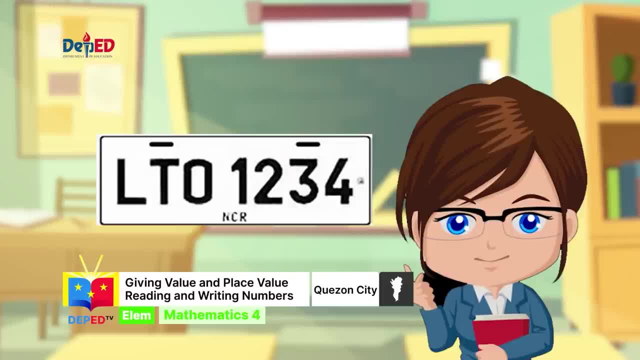 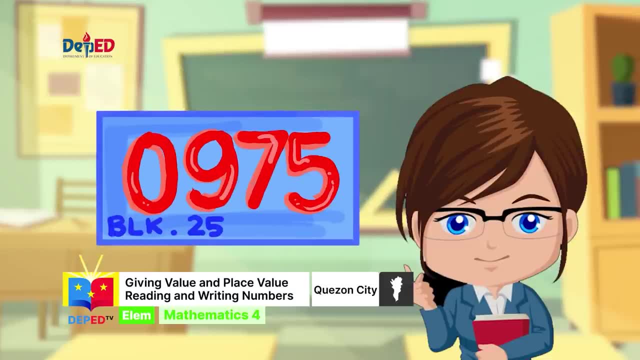 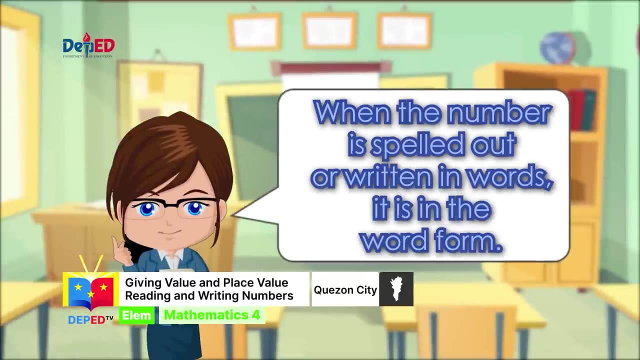 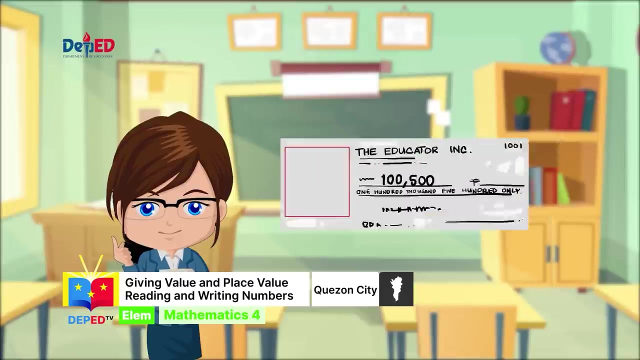 For example, plate numbers, Numbers in the calculator, The number of your house Dates in the calendar. On the other hand, the number is spelled out or written in words. It is in the word form. For example, we can see it in check vouchers and other important documents. 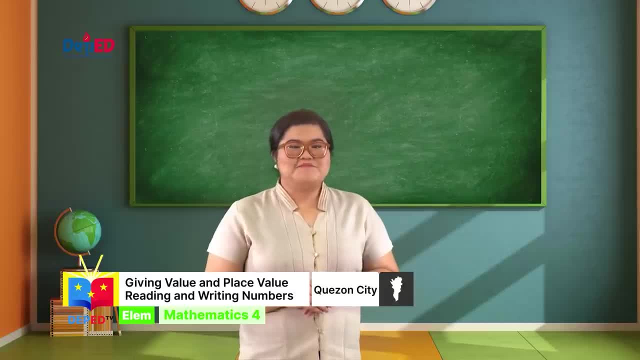 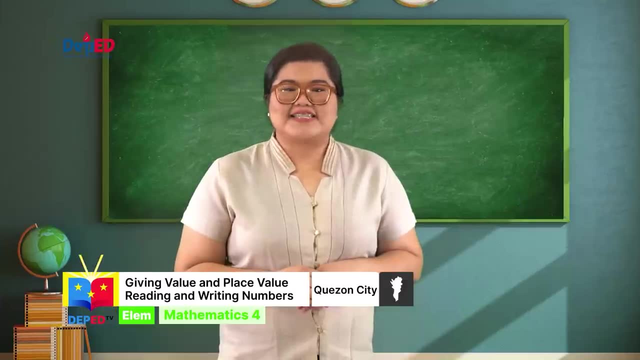 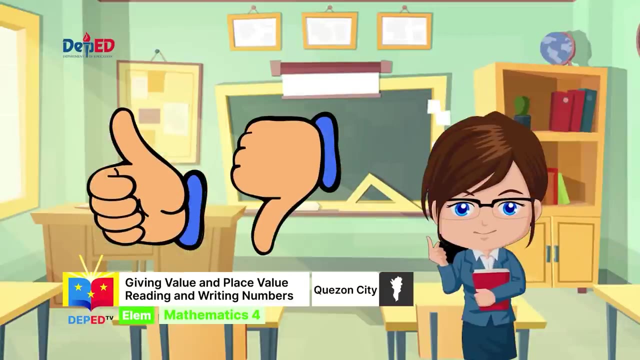 Math Galing, Math Galing, Math Galing. Practice time, Math Galing, Buddies ready. As long as Teacher Marian is with you, you can do it. Show me your thumbs. You will do thumbs up if the number is in standard form. 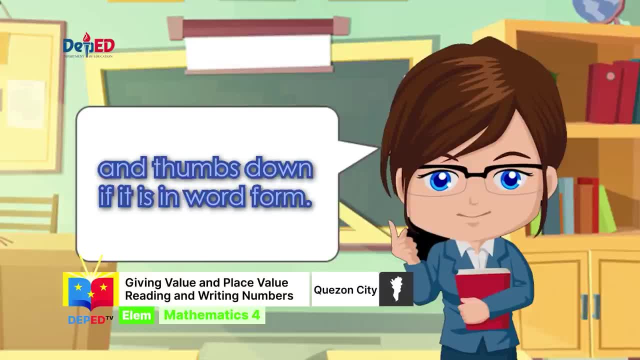 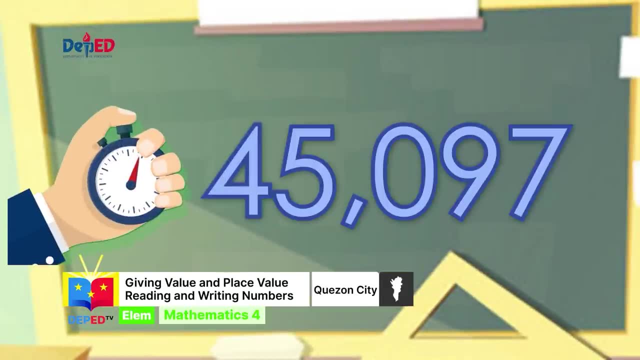 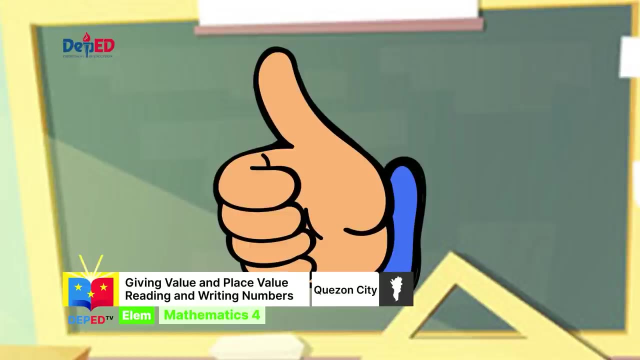 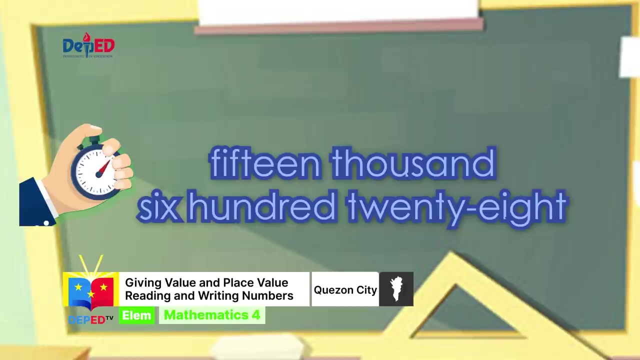 and thumbs down if it is in word form. You have five seconds to think for your answer Number one: Thumbs up or thumbs down. Okay, Thumbs up Next. Thumbs up or thumbs down. Correct, Thumbs down. 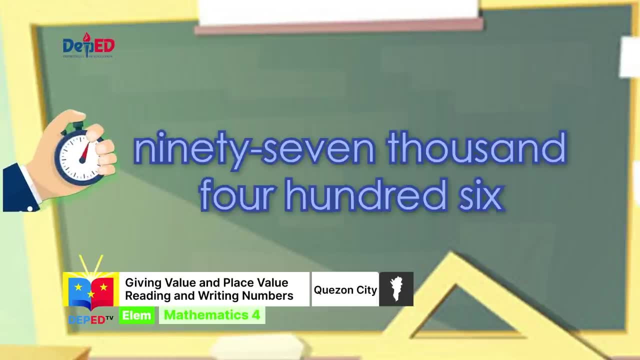 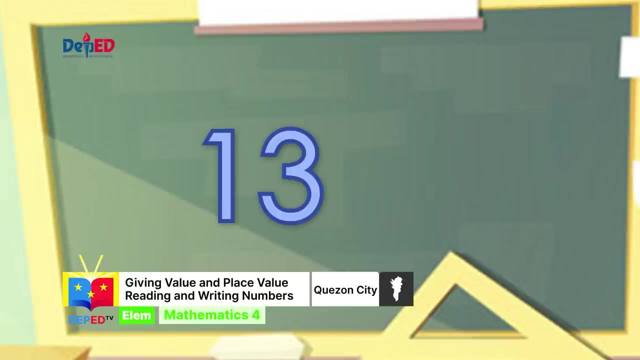 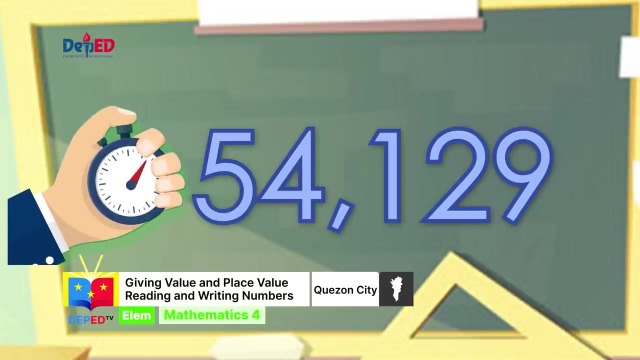 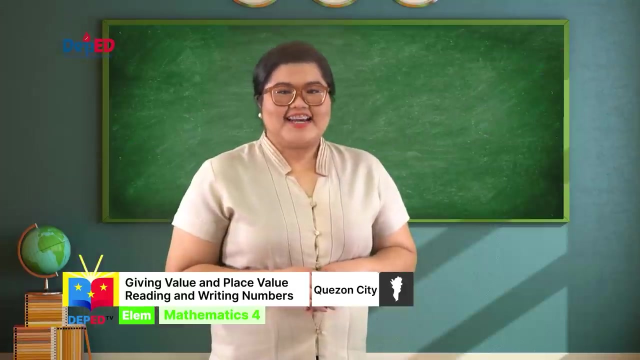 Number three: Thumbs up or thumbs down. Bravo, Thumbs down. Next Thumbs up or thumbs down. Nice job, Thumbs up. Last number: Thumbs up or thumbs down. Amazing Thumbs up. Remember to write numbers up to 100,000 in standard form. 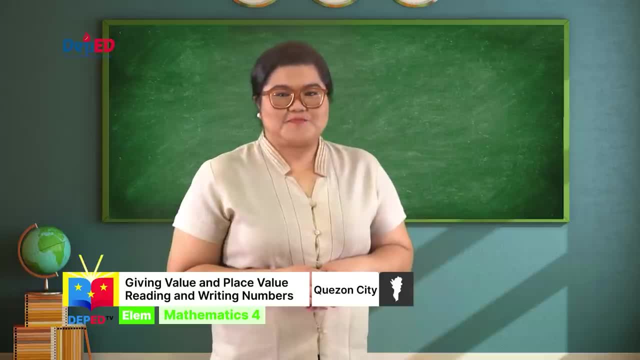 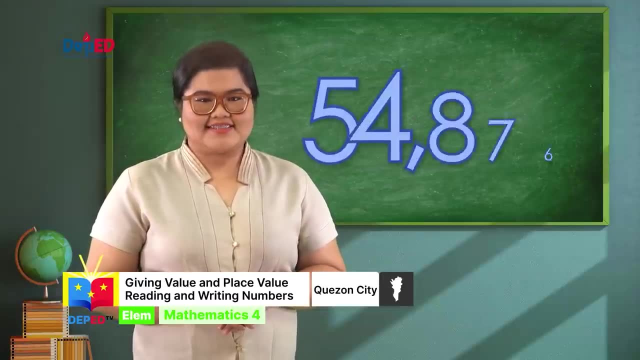 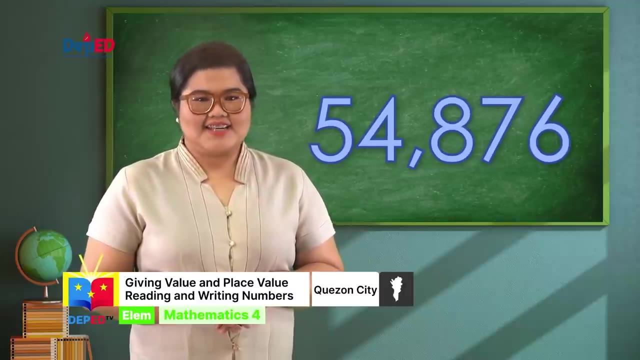 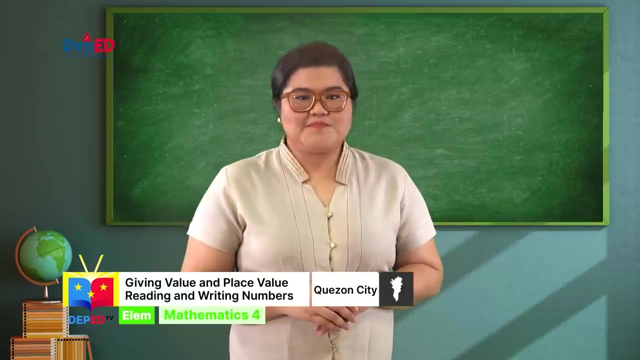 we use space to separate the digits into periods or groups of three, starting from the right. Let us try to read this number: Okay, 54,876.. When reading a number, always begin with the digits in the first period on the left and say the period where the digits are. 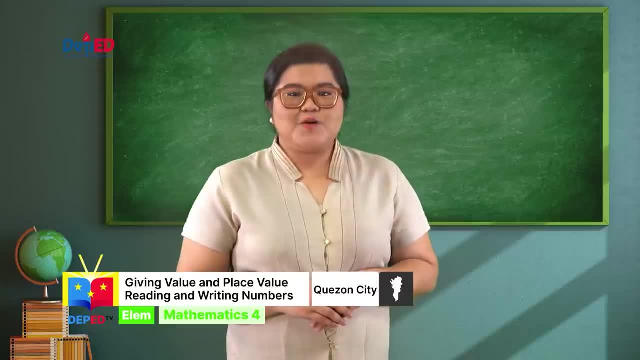 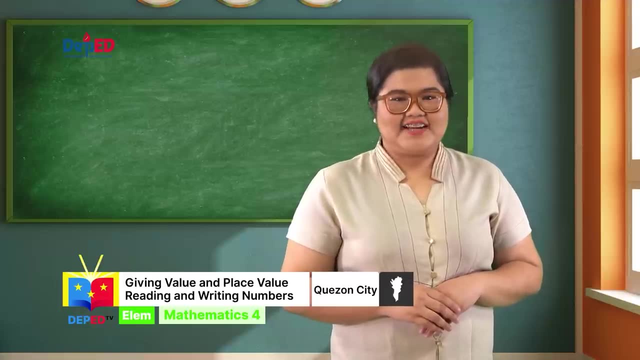 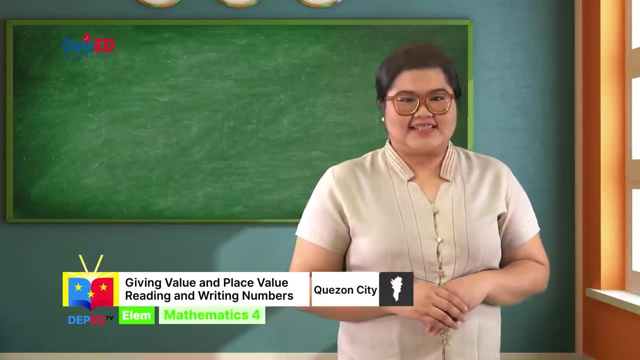 Do the same with a unit's period without saying the name of the period. Now let us write it in word form. Remember, we write the number the same way they are read, starting from left to right. So 54,876 is written as a number. 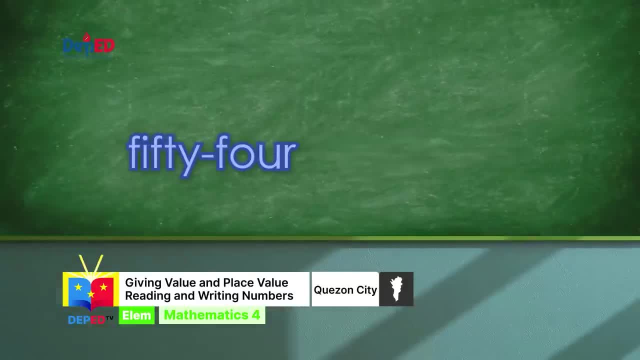 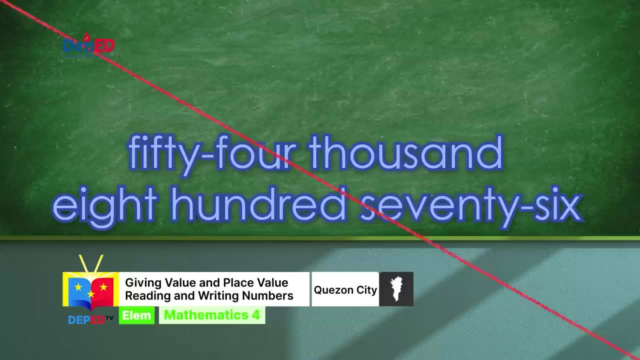 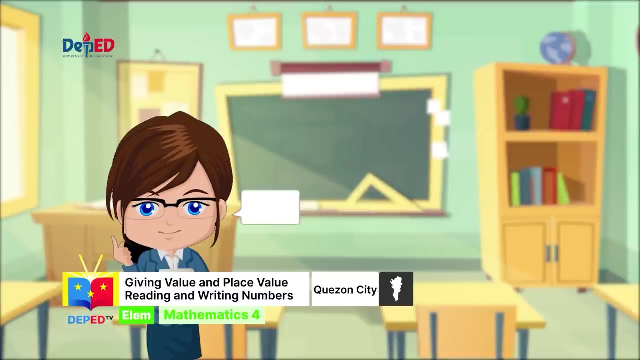 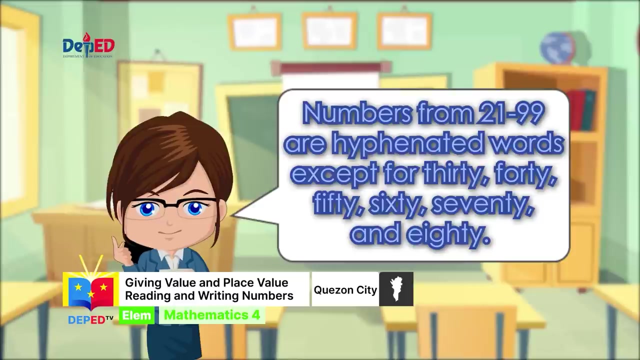 So 54,876 is written as a number. Have you observed there were hyphenated numbers? Don't forget that numbers from 21 to 99 are hyphenated words, except for 30,, 40,, 50,, 60,, 70, and 80. 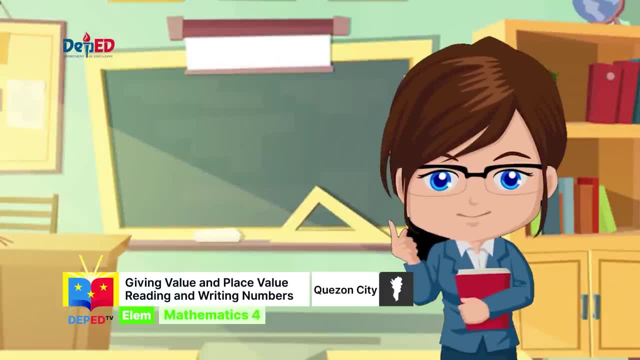 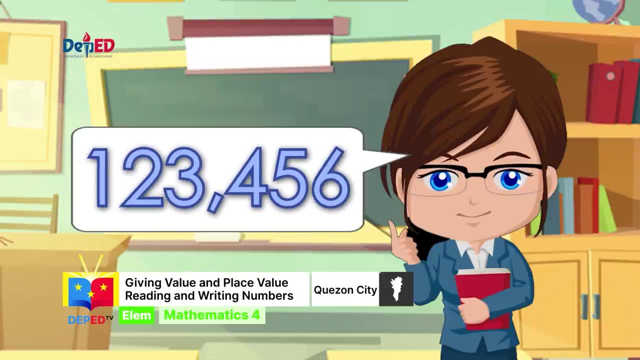 Except for 30,, 40,, 50,, 60,, 70, and 80.. Except for 30,, 40,, 50,, 60,, 70, and 80.. In writing. big numbers. we can use a comma or space to separate the digits into groups of three. 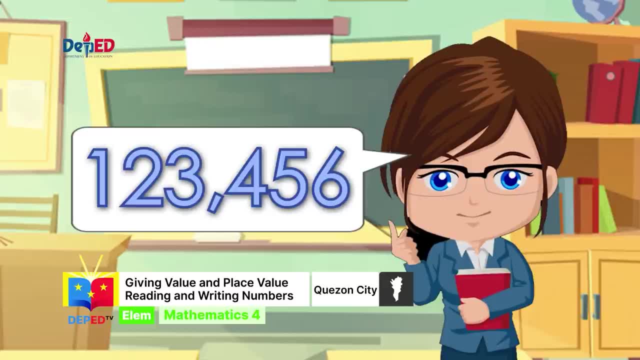 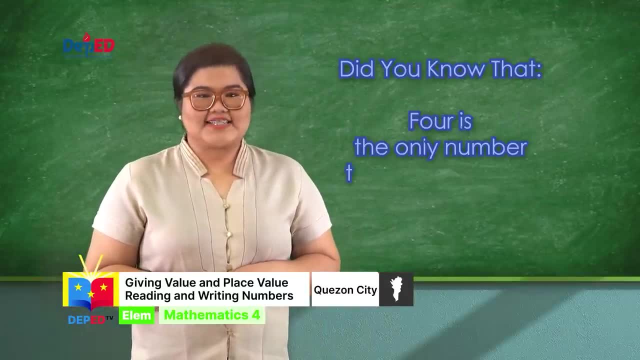 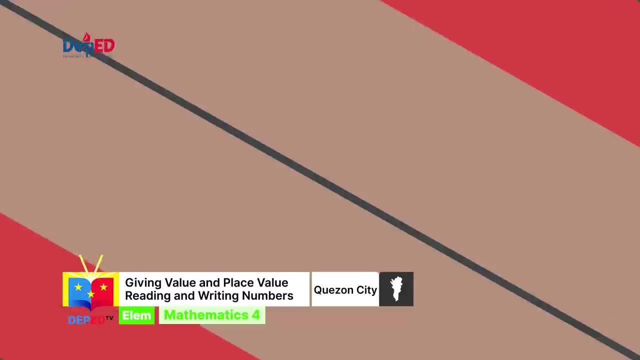 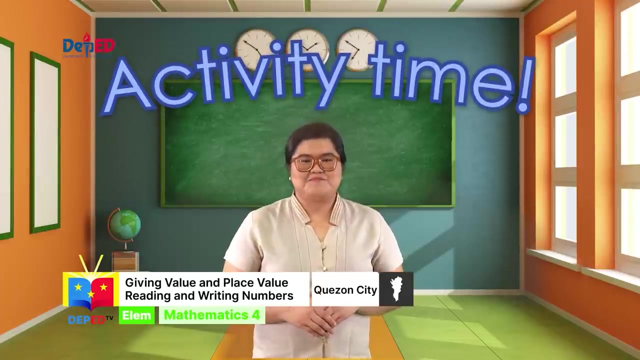 We can do this by counting three numbers from the right Trivia time. Did you know that four is the only number that has the same number of letters as its meaning? Mathgaling, Mathgaling. Activity time: Pens up- Papers up. 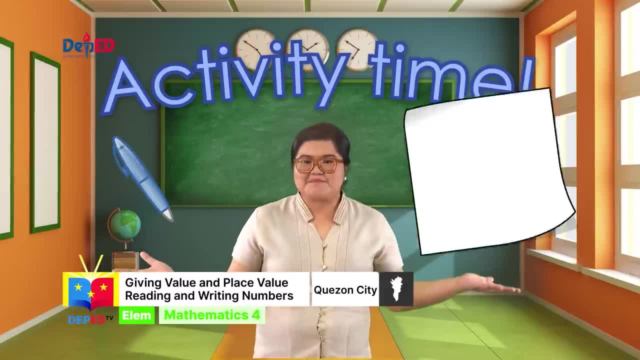 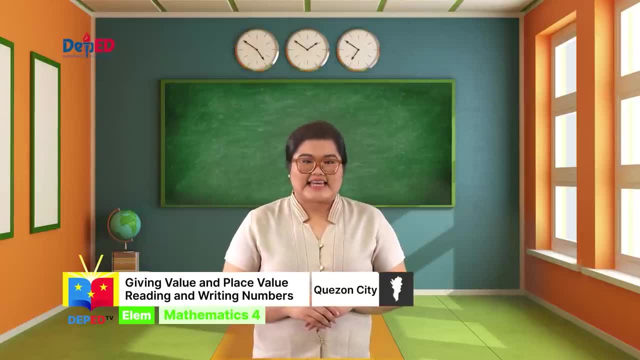 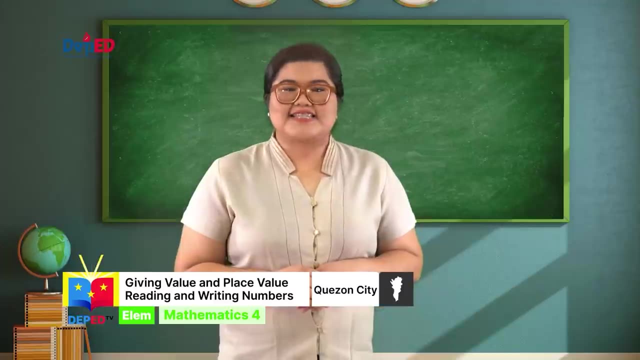 Let me see your happy face. Pens up, Papers up. Let me see that amazing face. I will give you 10 seconds to answer each number. Mathgaling buddies ready. As long as I'm with Teacher Marian, I can do it. 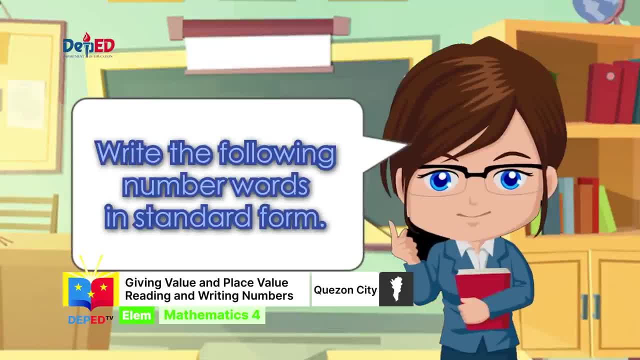 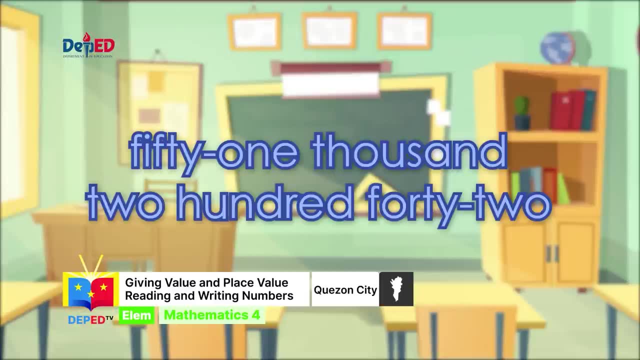 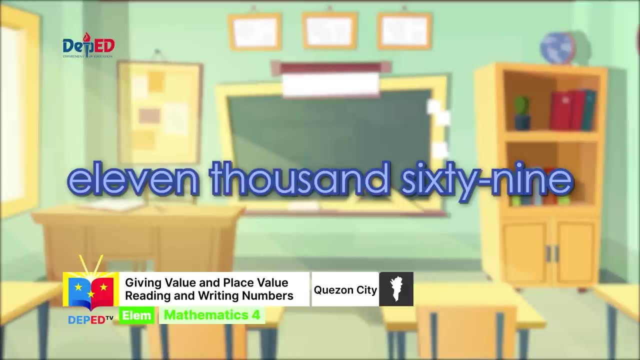 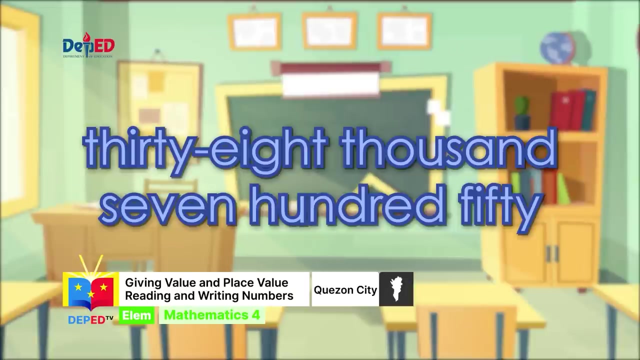 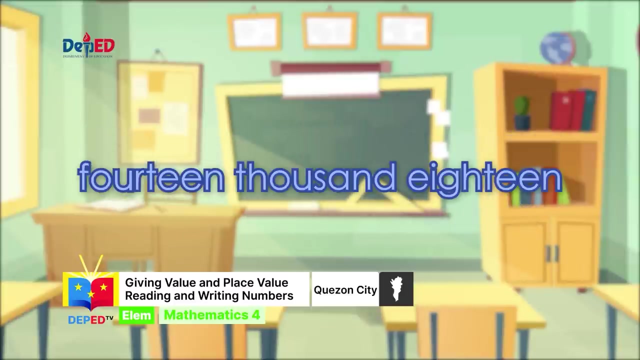 Write the following number words in standard form: Number 1, 51,242. Number 2, 11,069. Number 3, 38,750. Number 4, 14,000. Number 5, 90,900. Let's check your answer. 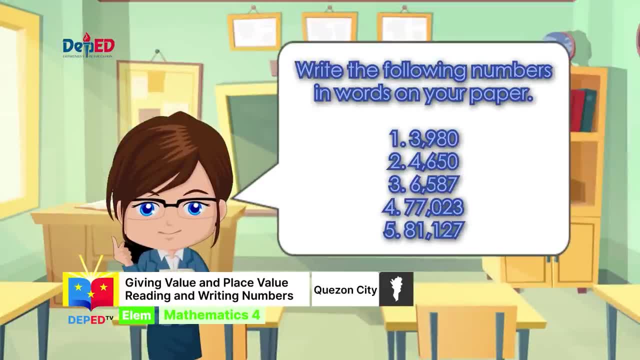 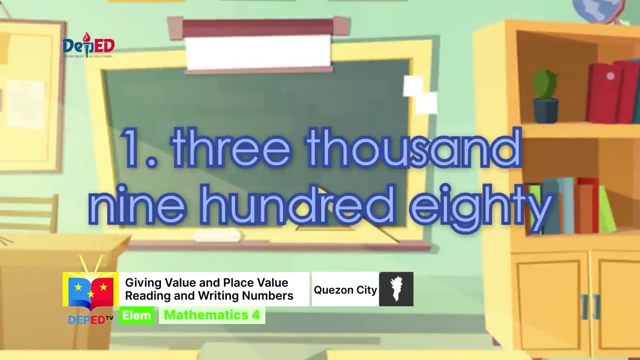 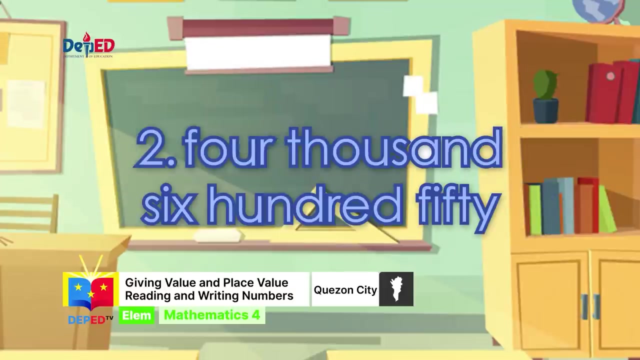 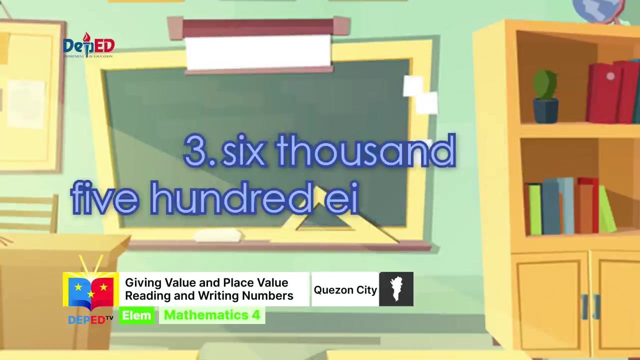 Next activity. Write the following numbers in words: Write the following numbers in words on your paper. Let's check your answer: Number 1, 3,980. Number 2, 4,650. Number 3, 6,587. Number 4, 77,023. 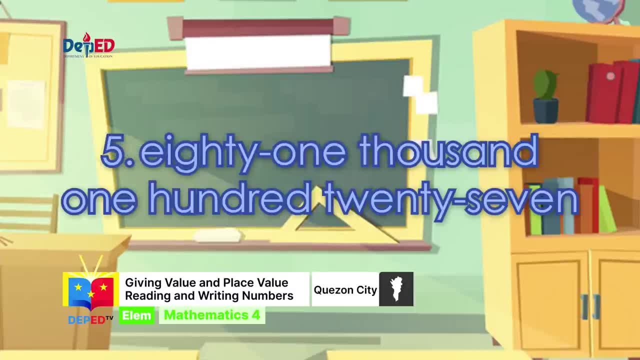 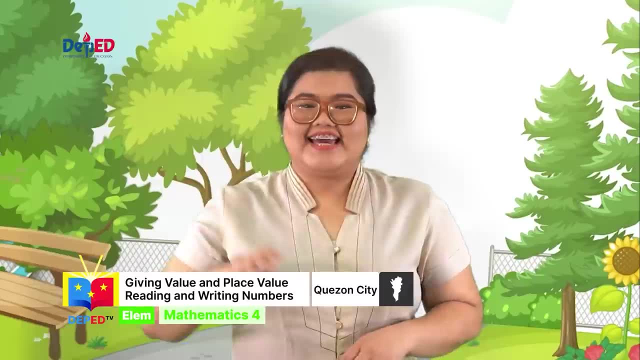 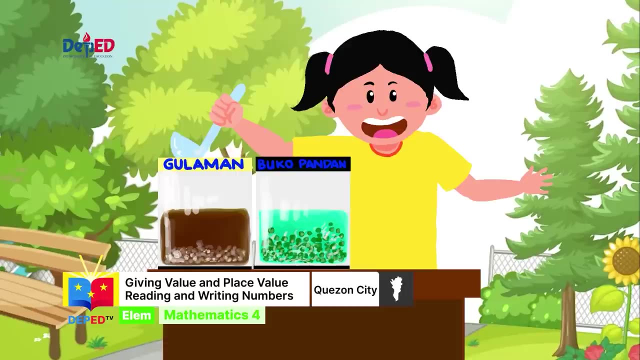 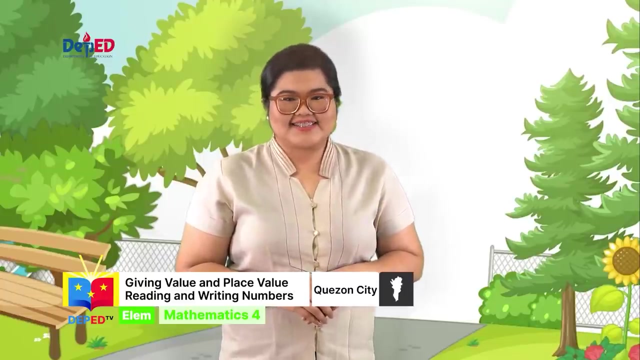 Number 5, 81,127. Number 6, 21,20,27. Hi Anna, It seems that you have added one more flavor. Yes, Teacher, Marian, I have kulaman flavor and buko pandan flavor. Kindly give me one glass of buko pandan drink. 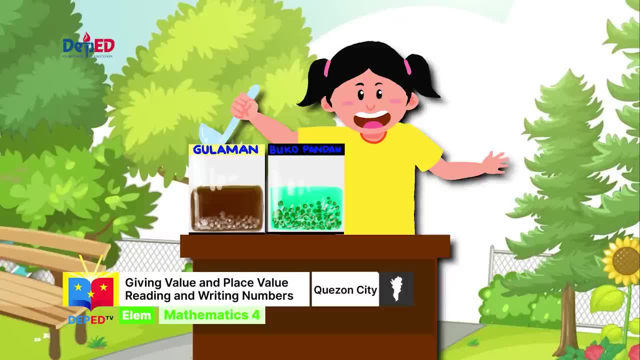 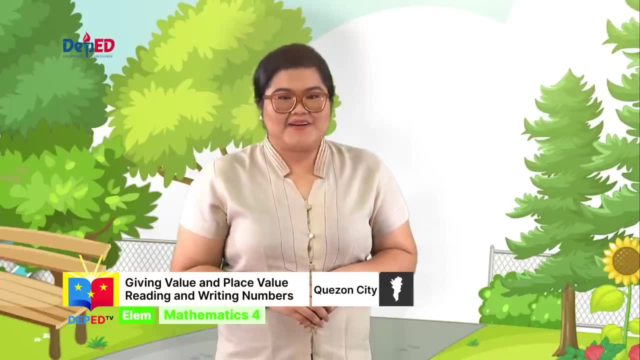 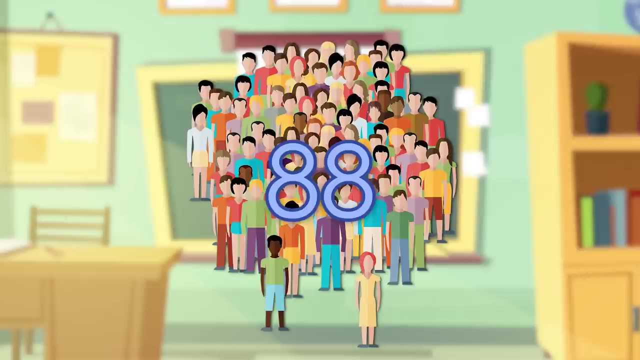 Sure teacher, Teacher, can you help me compare what drink is the most favorite of my customers? Sure Math, Galing Buddies, hop in, We will help Anna. In one week there were 88 customers who bought Gulaman juice. 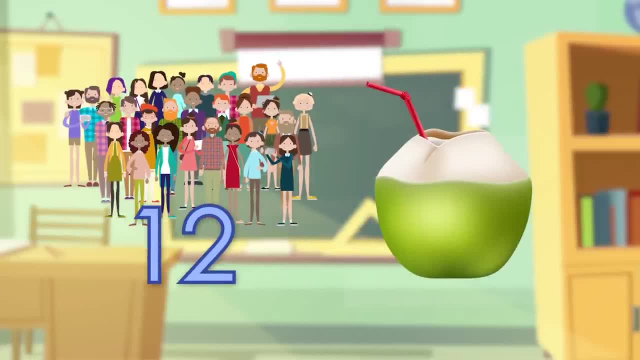 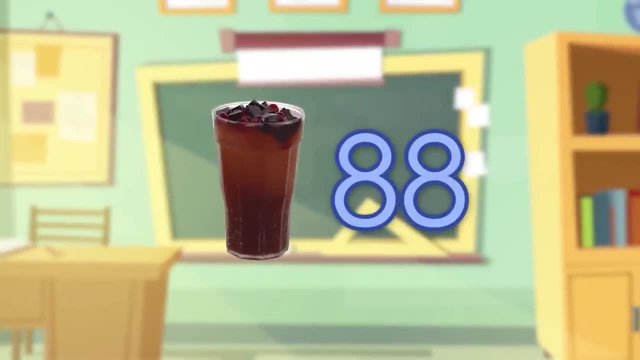 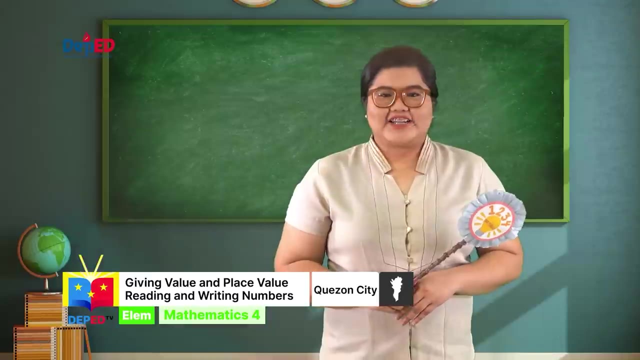 while 12 customers bought Buku Pandan juice. What is the best-selling juice of Anna Great Gulaman juice. We can say that 88 is greater than 12.. In comparing numbers, we are trying to find out which is bigger and which is smaller. 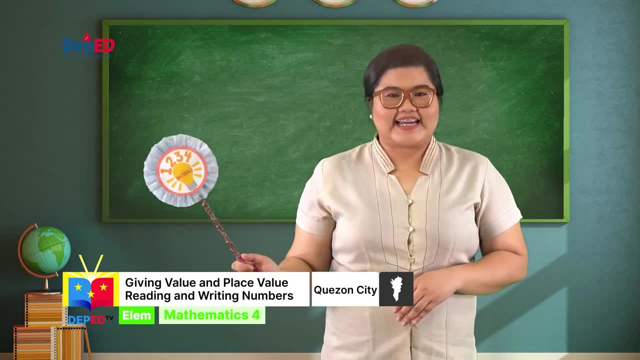 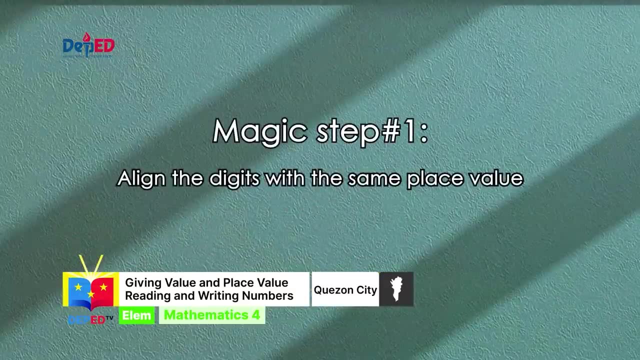 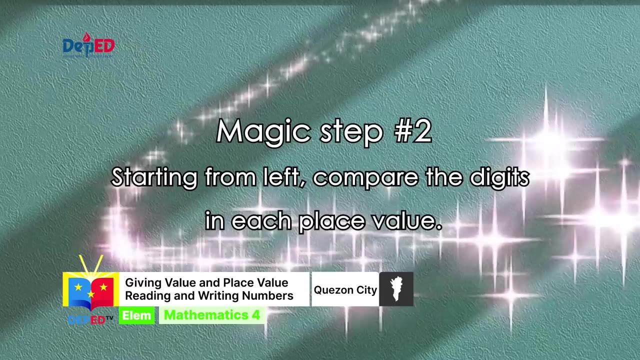 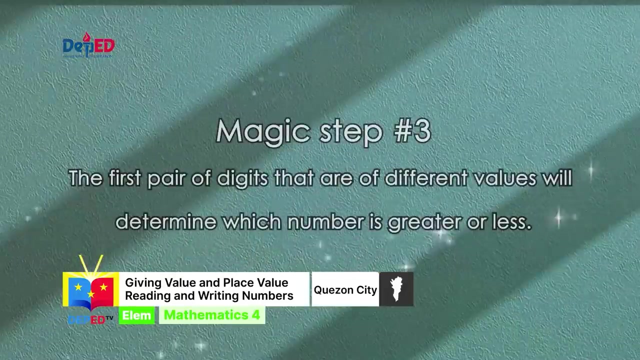 There are three magical steps in comparing two numbers. Magic Step Number 1.. Align the digits with the same place value. Magic Step Number 2.. Starting from left, compare the digits in each place value. Magic Step Number 3.. The first pair of digits that are of different values will determine which number is greater or less. 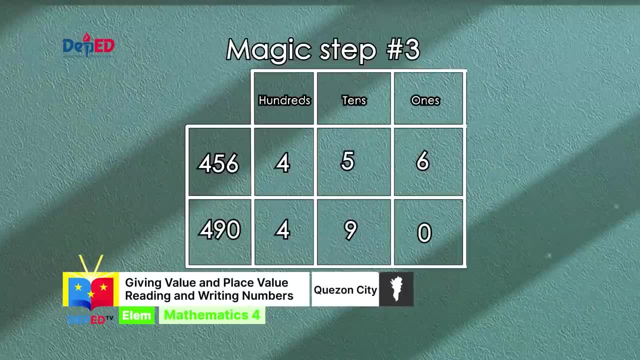 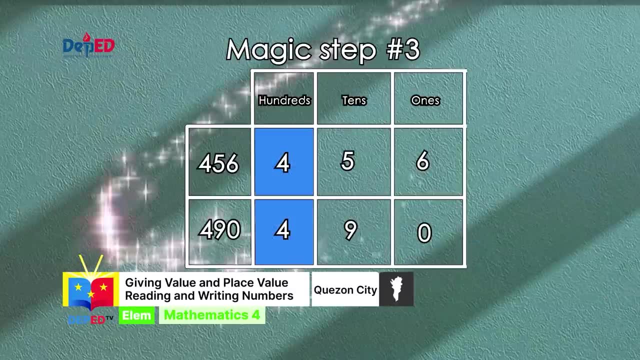 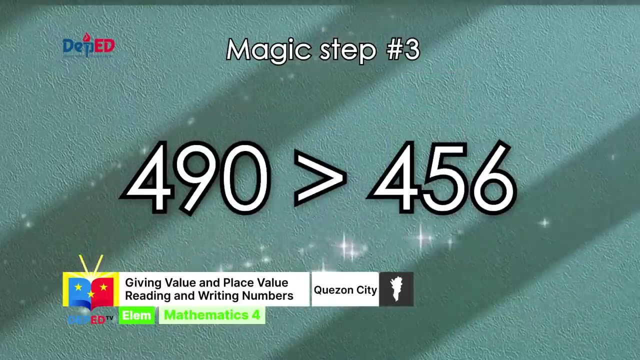 For example, study the table, The numbers have the same digit on the 100th place. On the 10th place, 9 is bigger than 5.. Therefore, 490 is greater than 400.. On the 11th place, 9 is bigger than 256.. 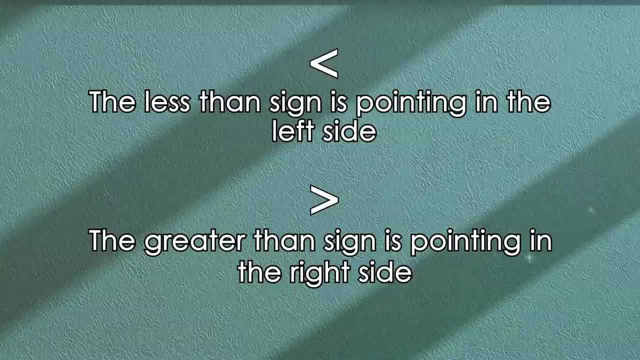 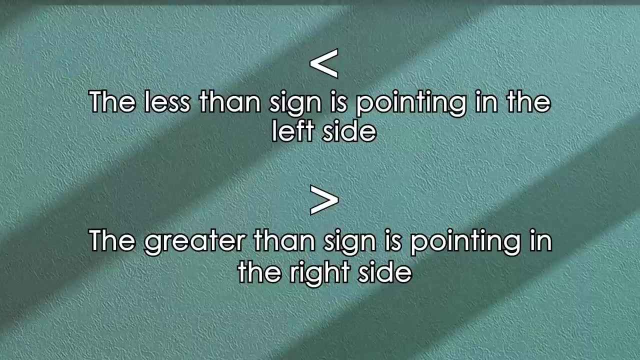 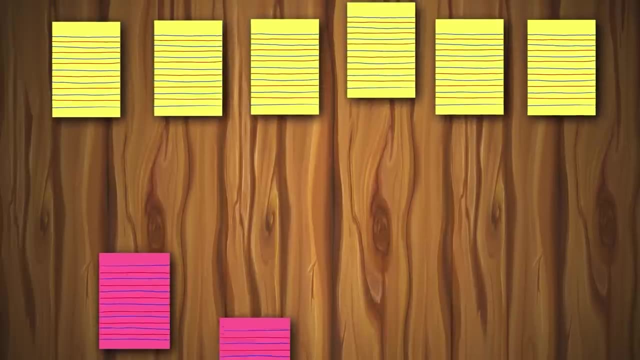 Let us review the symbols. in comparing numbers, The less than sign is pointing in the left side and the greater than sign is pointing in the right side. I have here different colors of paper. Let us compare each Number: 1. Yellow and pink. 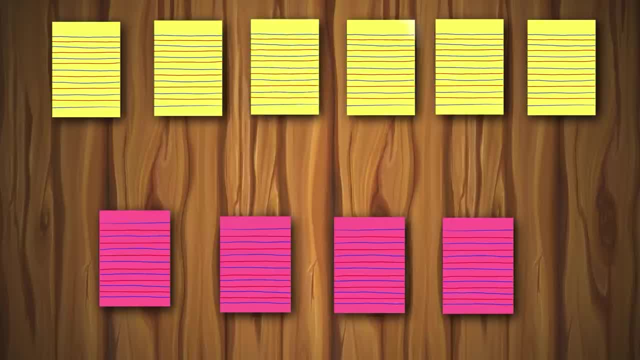 We have 1,, 2,, 3,, 4,, 5, 6.. We have 1,, 2,, 3,, 4,, 5, 6.. We have 1,, 2,, 3,, 4,, 5, 6.. 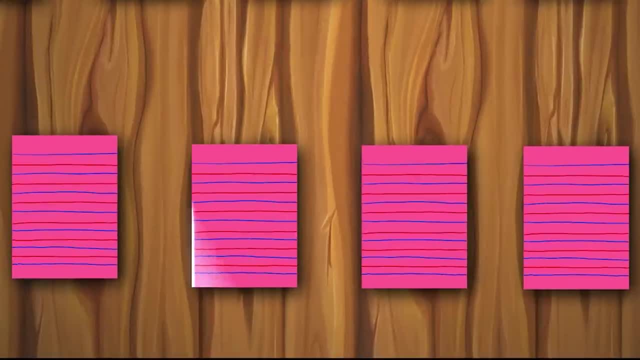 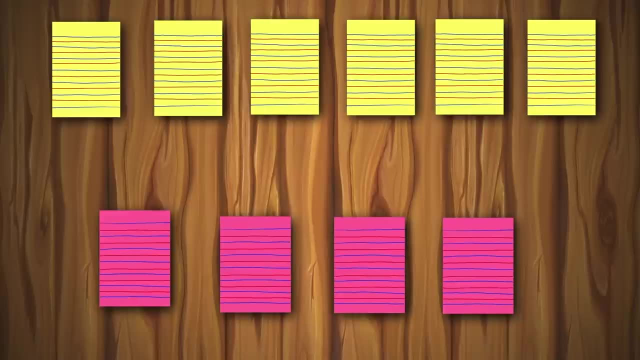 Yellow papers and 1,, 2,, 3,, 4 pink papers. Which is greater Yellow? We can say that 6 is greater than 4.. We will use the greater than symbol. The pointed part of the arrow is facing the smaller number. 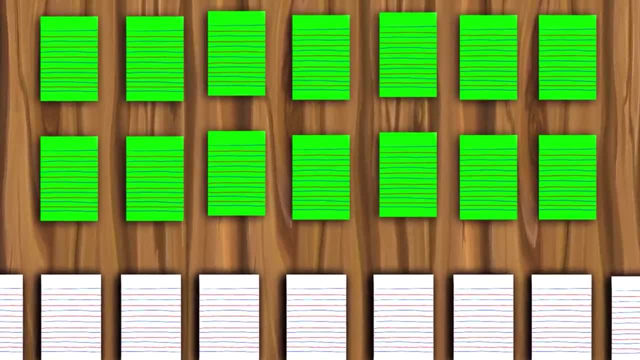 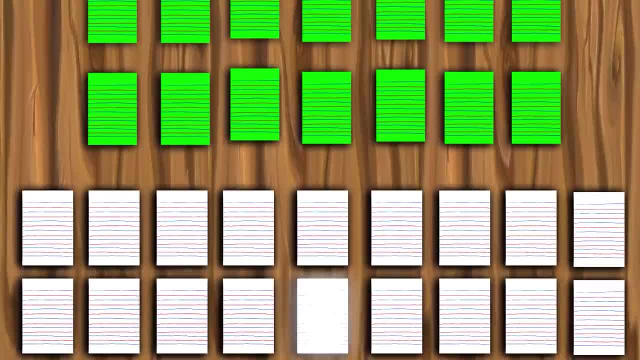 We have 1,, 2,, 3,, 4,, 5,, 6.. We have 1,, 2,, 3,, 4,, 5,, 6.. 4,, 5,, 6,, 7,, 8,, 9,, 10,, 11,, 12,, 13,, 14,, 15,, 16,, 17, and 18 white papers. 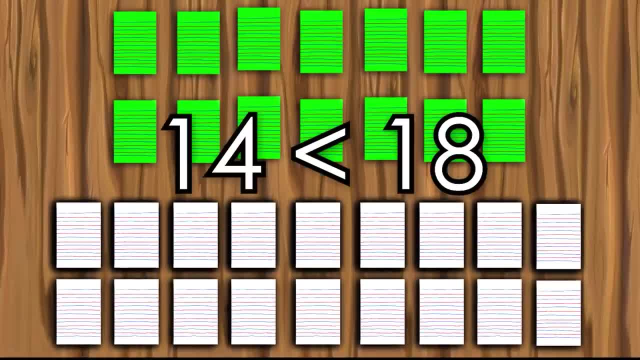 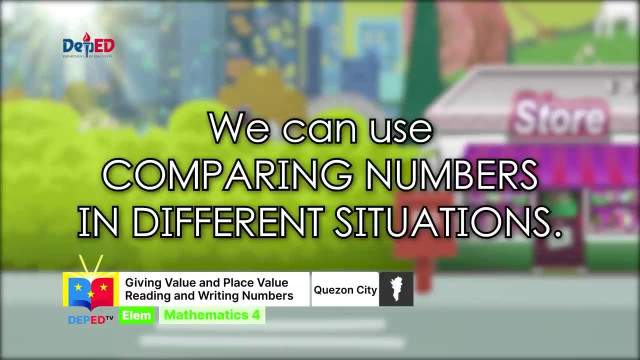 The green papers are less than the white papers, 14 is less than 18.. The pointed part of the arrow is facing the smaller number. We can use comparing numbers in different situations. Number 1. In going to the store, your mom asked you to buy cooking oil. 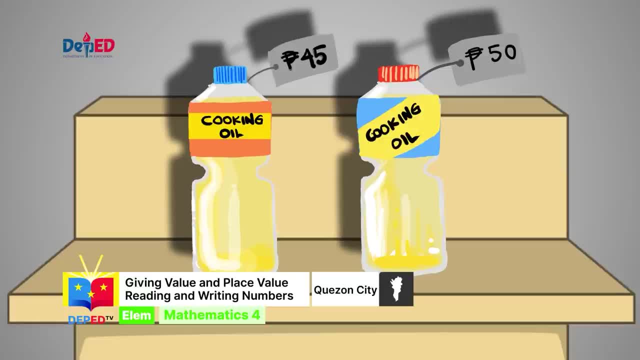 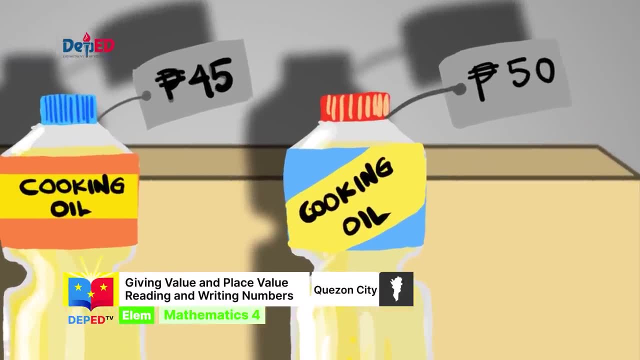 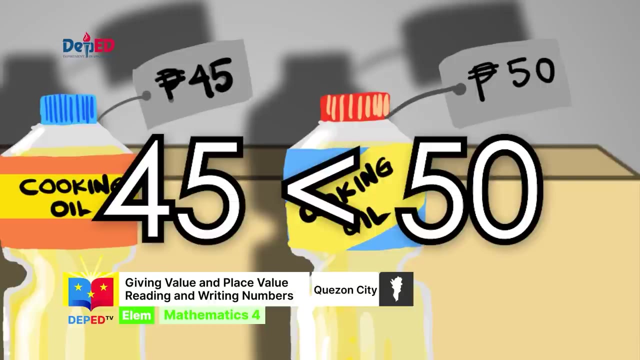 There were two prices of different cooking oil and your mom told you to choose the cheapest price. What should we buy? Yes, the 45 peso cooking oil, because 45 is less than 50.. Number 2. In singing in a karaoke. 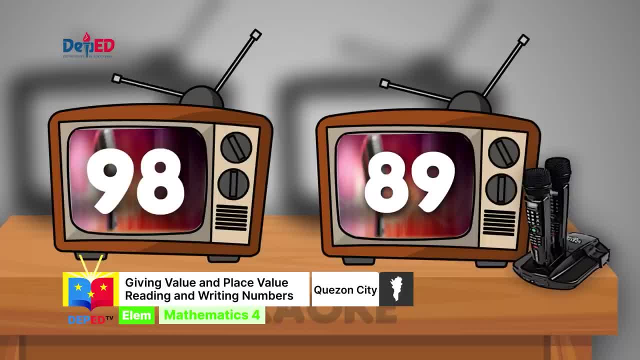 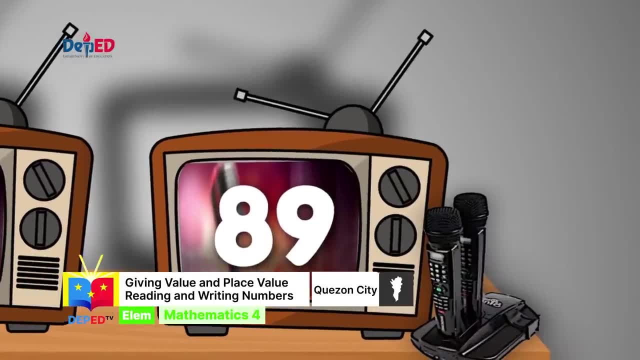 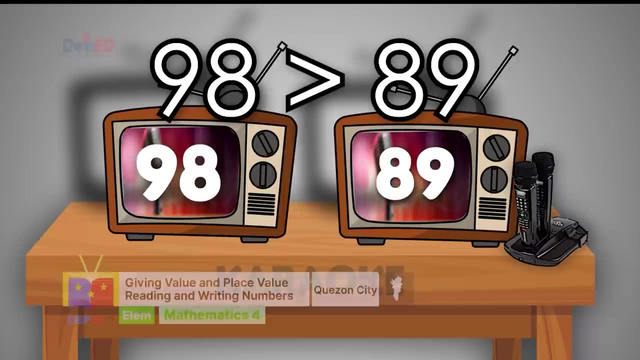 When you and your friend compete, who will have the highest score? You scored 98 and she scored 89. Who is the winner? Of course, 98 is greater than 89 and you are the winner. Math galing, math galing, math galing. 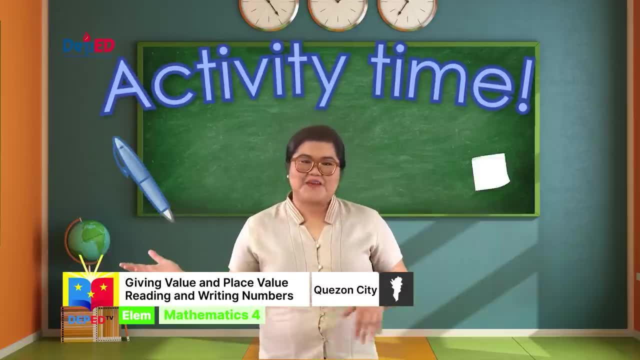 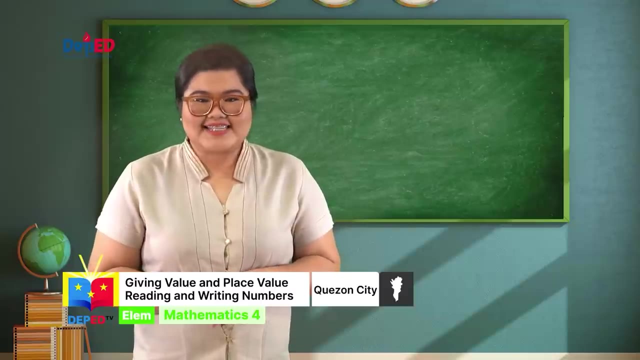 Activity time. Tense up papers up. let me see your happy face. Tense up papers up. let me see that amazing face. I will give you 10 seconds to answer each number. Math galing buddies ready. Basta kasama si Teacher Marian kaya yan. 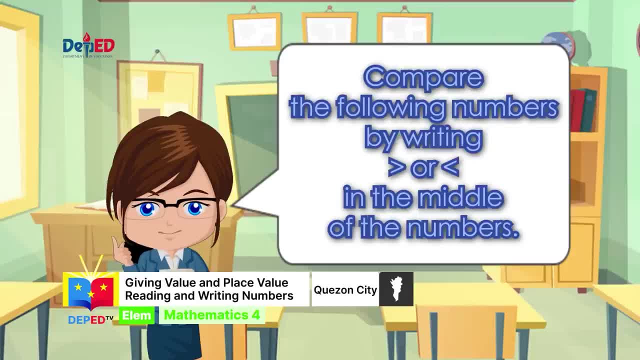 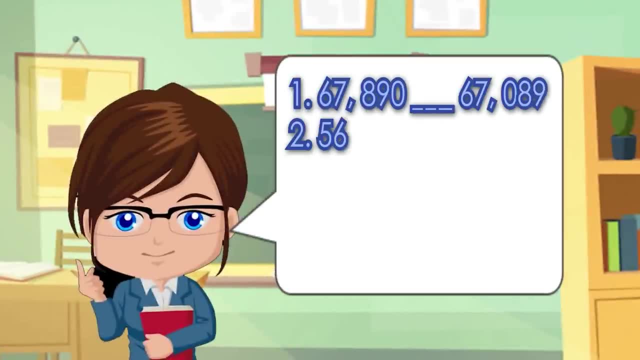 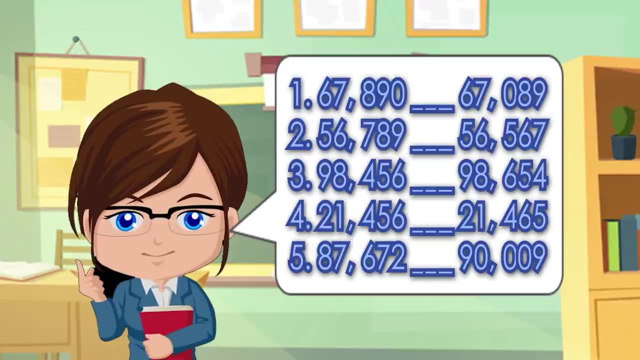 Compare the following numbers by writing greater than or less than in the middle of the numbers: Number 1, 67,890.. 67,089.. Number 2, 56,789.. 56,567.. Number 3, 98,456. 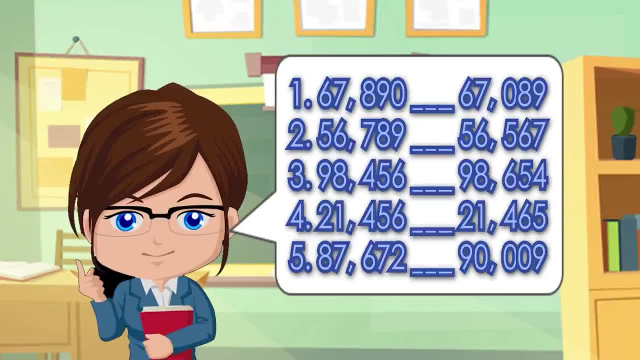 98,654.. Number 4, 21,456.. 21,465.. And number 5, 87,672.. 90,009.. Number 3, 87,632.. 90,009.. Number 4, 28,322.. 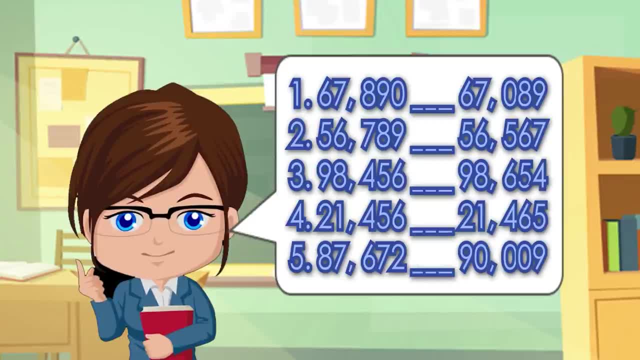 And number 5, 87,672.. 93,921.. Number 4, 20,200.. Number 2, 39,220.. Number 4, 20,200.. Number 3, 39,220.. 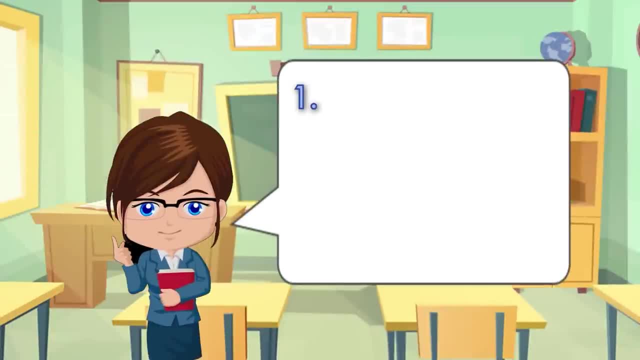 Number 4, 2000.. Let us answer: Number 1, 67,890 is greater than 67,089.. Number 2, 56,789 is greater than 56,567.. Number 3, 98,456 is less than 98,654.. 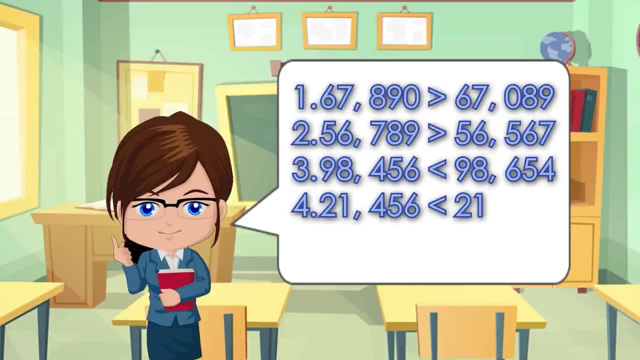 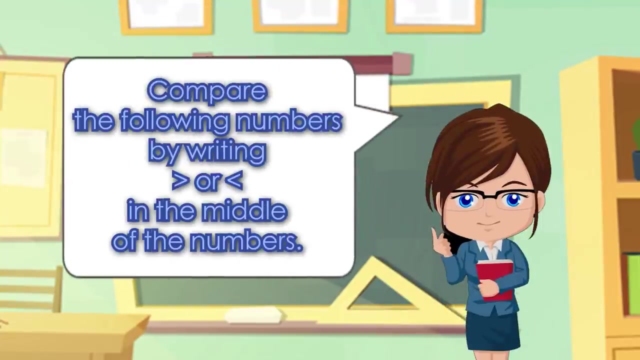 Number 4, 21,456 is less than 21,465.. And number 5, 87,672 is less than 90,009.. Let's have another activity. Compare the following numbers by writing greater or less than on the middle of the numbers. 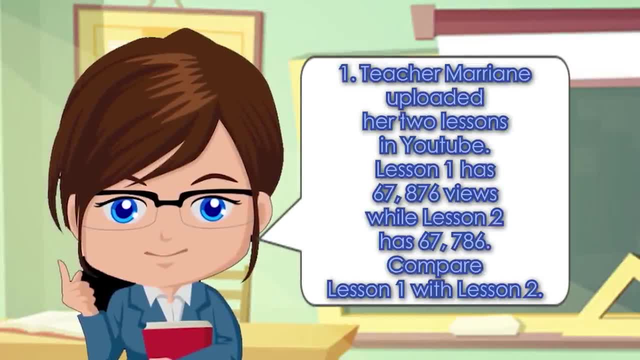 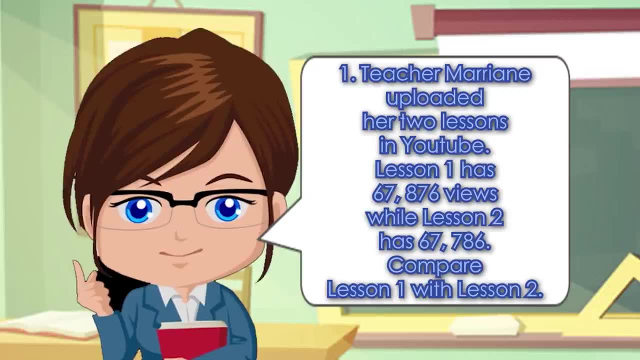 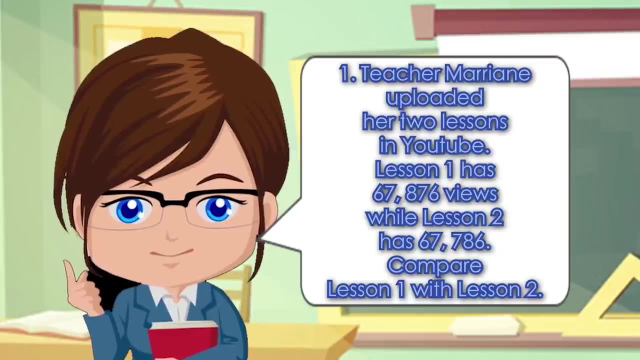 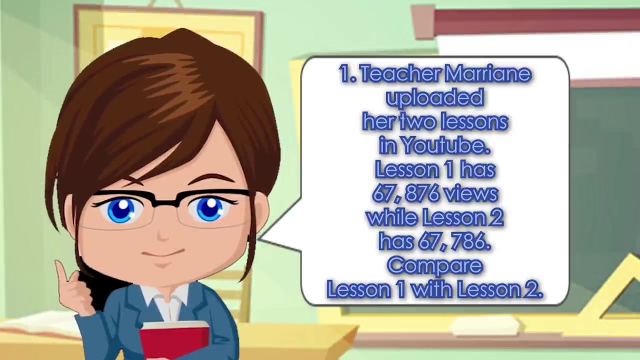 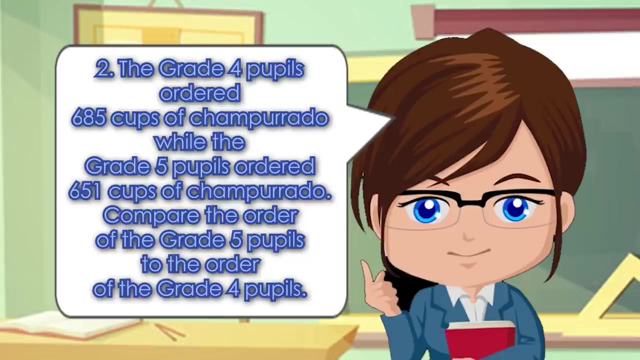 Number 1, Teacher Marian uploaded her two lessons in YouTube. Lesson 1 has 67,876 views, while Lesson 2 has 67,786.. Compare Lesson 1 to Lesson 2.. Number 2, the grade 4 pupils ordered 685 cups of Ciampurado, while the grade 5 pupils ordered 651 cups of Ciampurado. 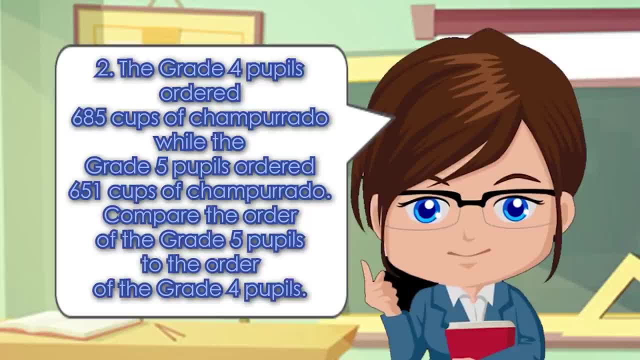 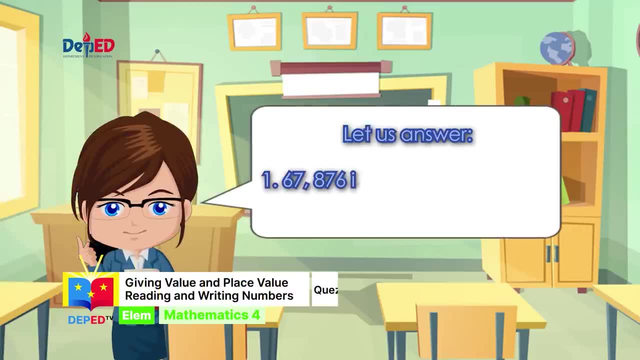 Compare the order of the grade 5 pupils to the order of the grade 4 pupils. Let us answer: Number 1, 67,876 is greater than 67,786.. Number 2, 651 is less than 685.. 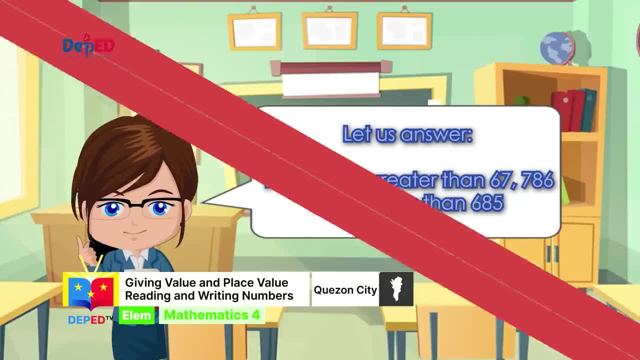 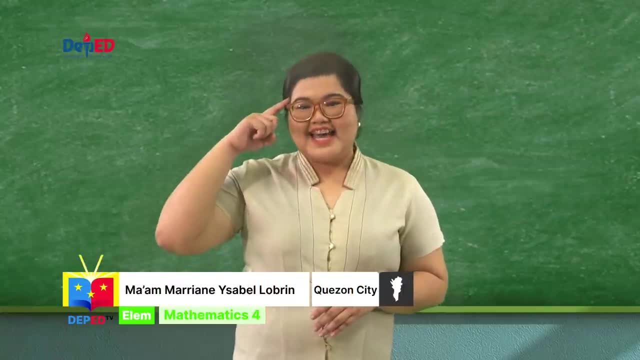 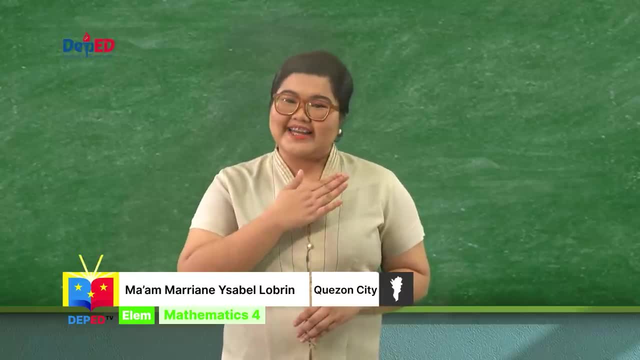 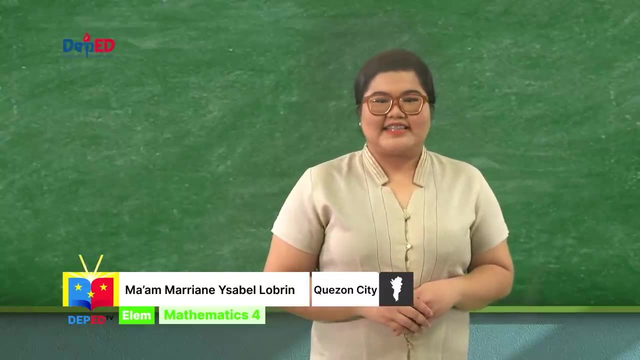 Keep this in mind. The best way to learn mathematics is to learn math. Remember, as long as Teacher Marian is with you, you can do it. That's it for today. Math Galing Buddies, See you on our next math-exciting and math-amazing activities. 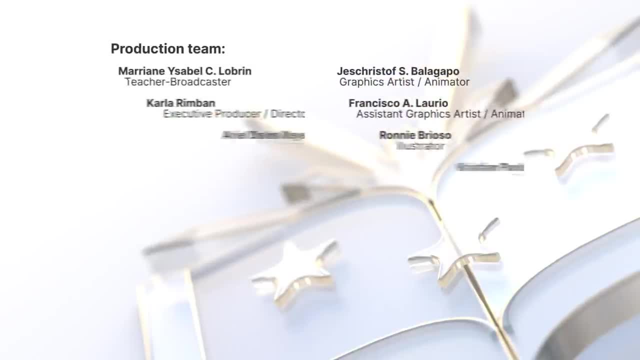 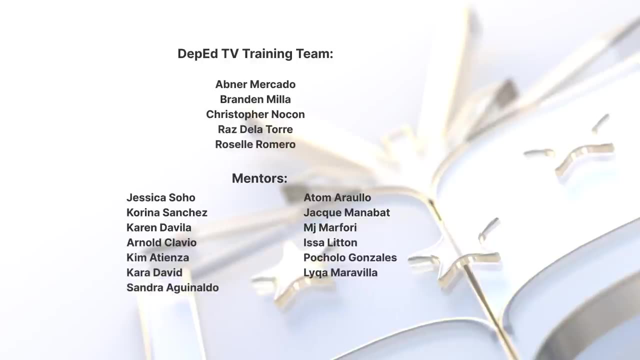 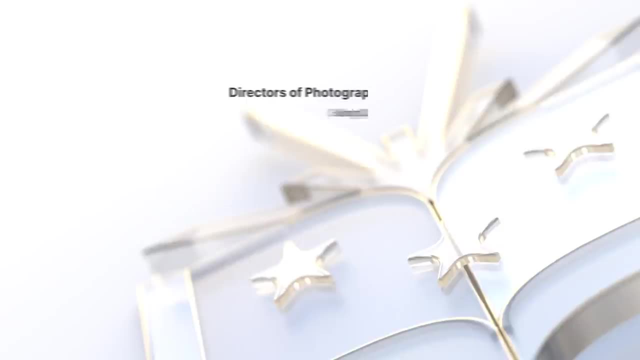 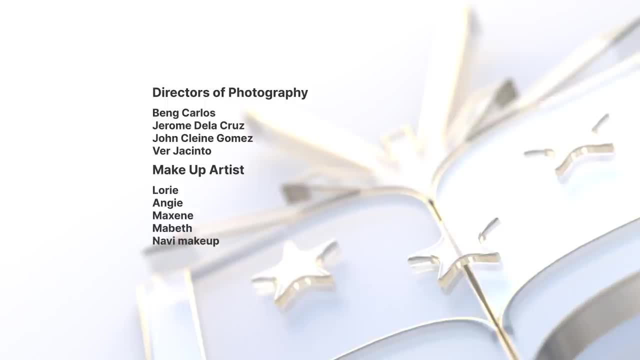